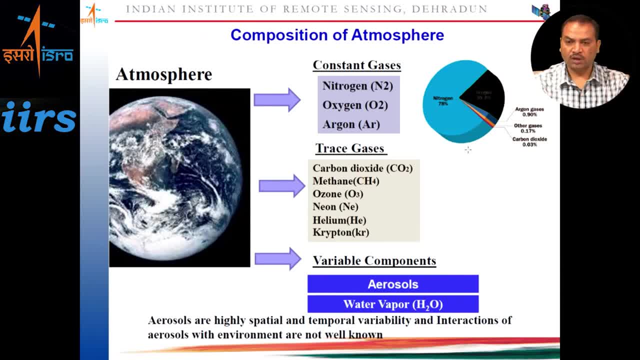 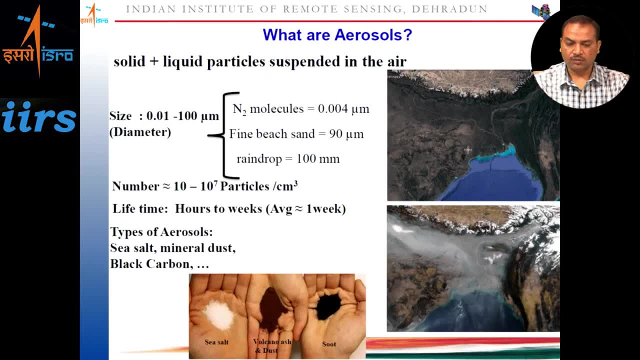 variability. So they have these variable components. So these are the aerosols. So, and they have quite good interaction and with the optical and physical properties, with the environment. Now, what are these aerosols? Now we are focusing our lecture on aerosols. 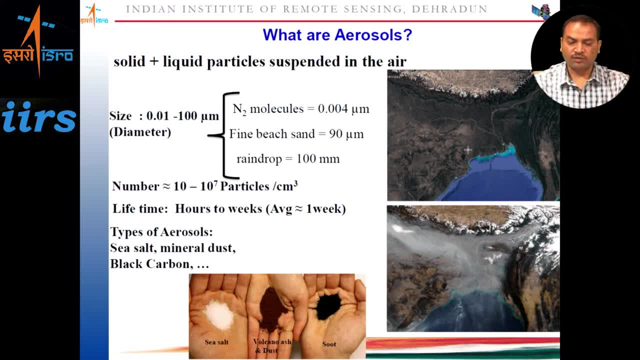 The aerosols are any solid or liquid particles which is suspended in the air. Now you must be knowing that the particle size of the molecules is very, very low. that is 10 raised power minus 7 minus 10 raised power minus 6 meter. Here I have given the nitrogen molecules 0.004. 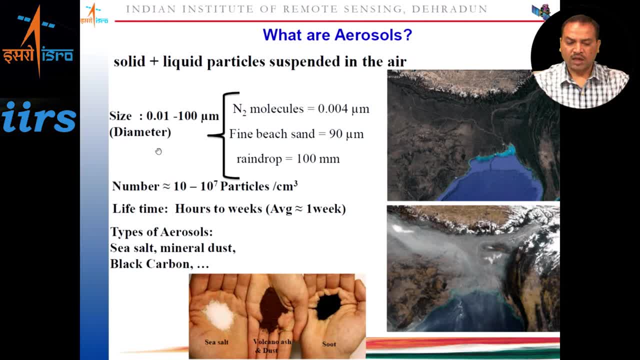 microns. The size of the aerosols are slightly larger than the gas molecules, which are in the size of 0.01 to 100 microns and the less than the raindrop size. small raindrop is 100 nanometer, So these are some of the size of the aerosols. So these are some of the size of the aerosols. 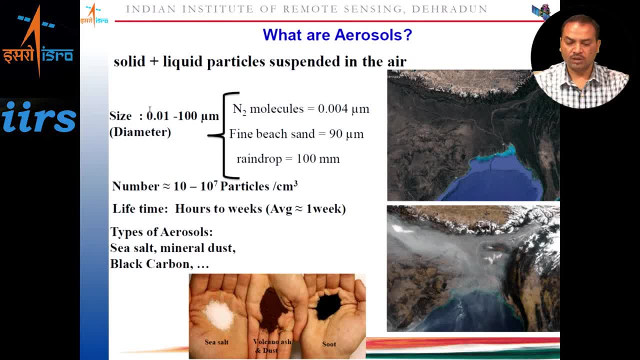 So these are some of the size of the aerosols: 0.01 to 100 micrometer. They also vary in the number density, that is, the particles per meter per meter square, per meter centimeter in the atmosphere. So 10 to the 10 raised power, 7 number density. So the fine. 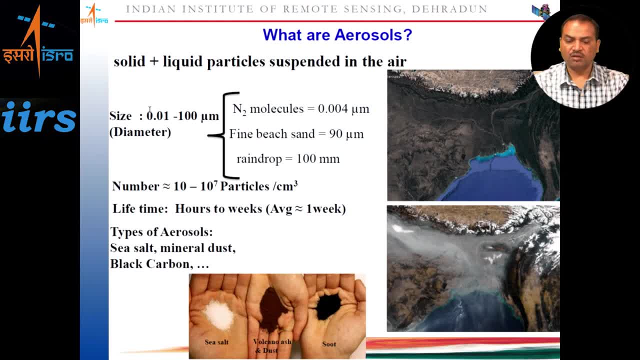 particles or the larger particles. they vary in the number, density in the atmosphere, and also they vary in terms of the lifetime, that is, when they are evolved or formed from the sources, how long they stay in the atmosphere, and then there is a decay with very. there are various. 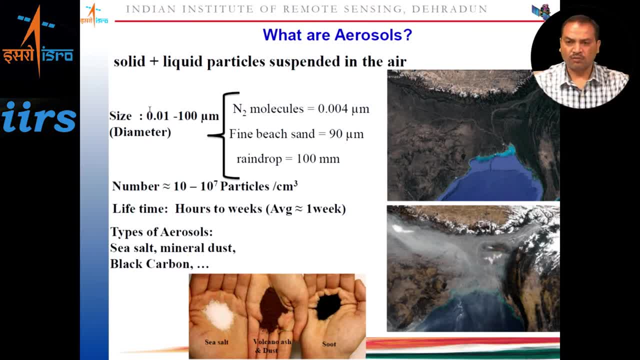 processes. So it is very low from hours to weeks. and when it goes to the upper layer in the stratosphere maybe it goes for months or maybe some years, but there are very few particles and when we talk about the type of…. 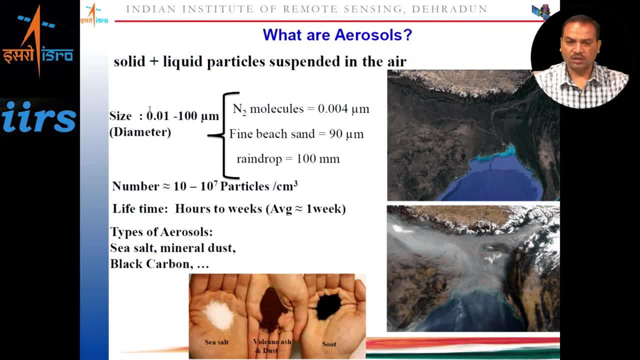 aerosols. as you know, that sea salt, the largest is the- 70 percent. 75 percent is the ocean and the the sea salt spray which is formed from the wind blown from over the sea surface, the sea salt, the mineral dust, the black carbon, the and etc. etc. as you see in the, the, the picture of the sea salt, sea salt. 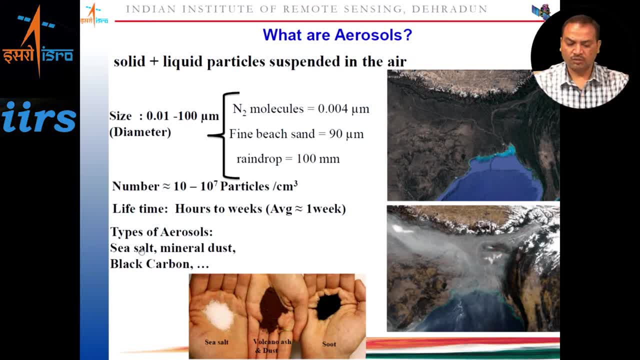 is larger in the size diameter of the aerosol and the volcanic ash or dust. and you see the suit. suit is the elemental carbon and these most of the aerosols are a scattering in nature and the anthropogenic that is a suit or element. carbon is having an absorption in nature. 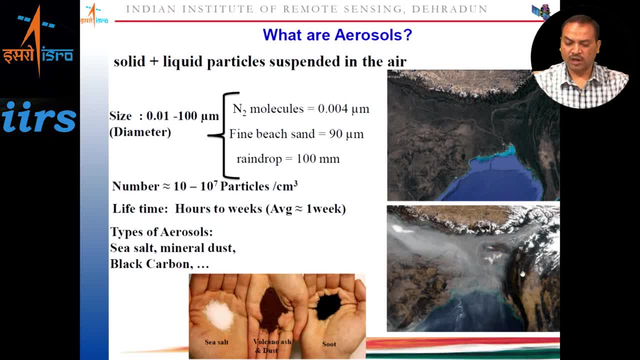 and you see that the eastern, the indo-gangetic plane and the bay of bengal region. it is filled with lot of aerosols or the. the anthropogenic emissions are clearly seen from the satellite image. and if you see the upper, the top image, it is a clear image with not such of 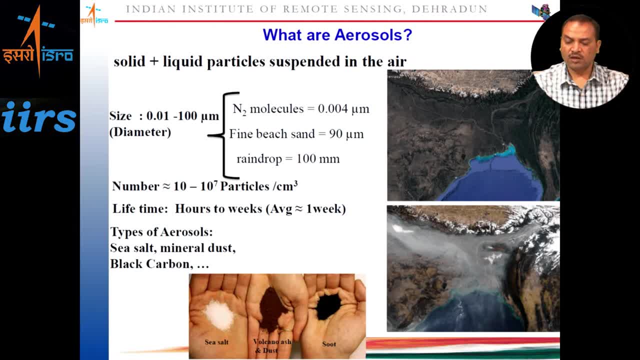 clouds or aerosols. so it means that there are, there are many sources, natural or the anthropogenic sources, which are responsible for many processes happening over the ocean or the land, and they, aerosols, stay there and it it also interact with the, the local weather and the particles and then 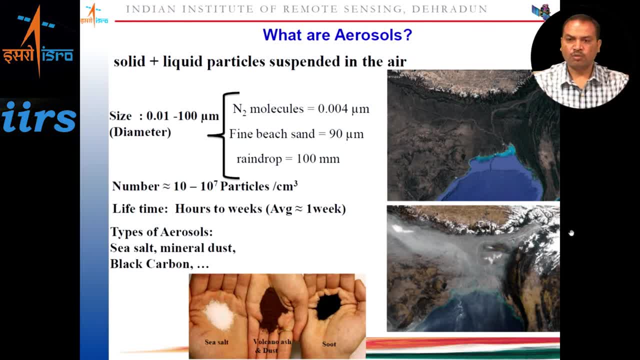 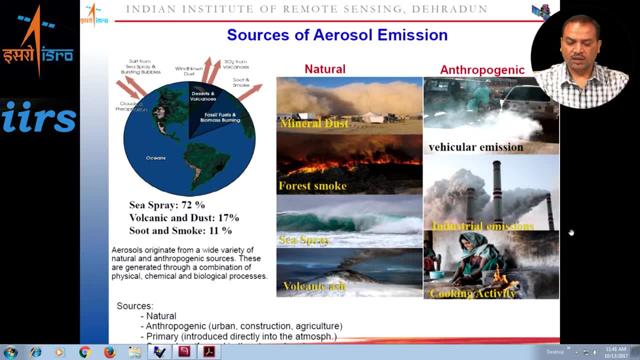 it leads to the many, many processes and effects. in terms of the sources of aerosols, as i said, the aerosol originate from a wide variety of natural and anthropogenic sources and it is formed through a combination of your physical, chemical and your biological processes. if you see that, you can. 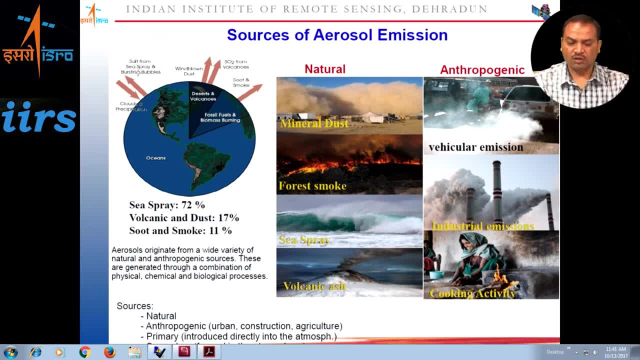 natural. natural comes sea salt, sea salt sprays around 72 percent. so the natural sources are sea salt. you are the volcano, volcanic, and dust and the and and the burning that is the natural burning. maybe may the forest fires the natural burnings. so all these, all these forms, the, your natural aerosols. 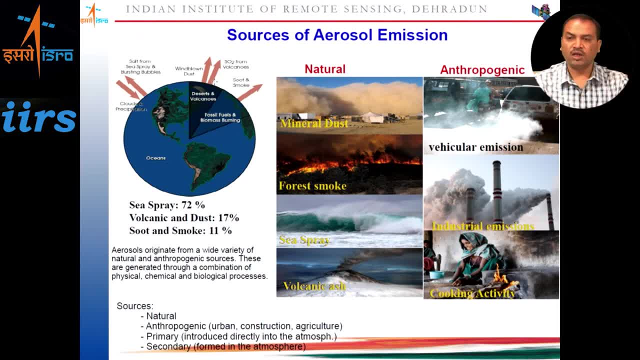 in terms of the anthropogenic aerosol. the sources are your urban and industrial emissions, the domestic fire combustions, and then the agriculture residue burnings, then the deforestation and then your land management practices, because lot of fertilizers and other things are used, so a lot. 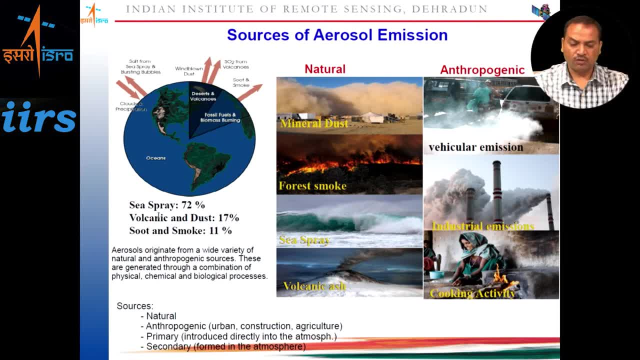 of land management practices are there and, of course, the wind erosions are also the the factors for the anthropogenic emissions. the these these are also divided into primary primary sources- are directly emitted in the atmosphere and and there are certain particles which react in the atmosphere and then leading to the secondary formation of the particles which lead also to the 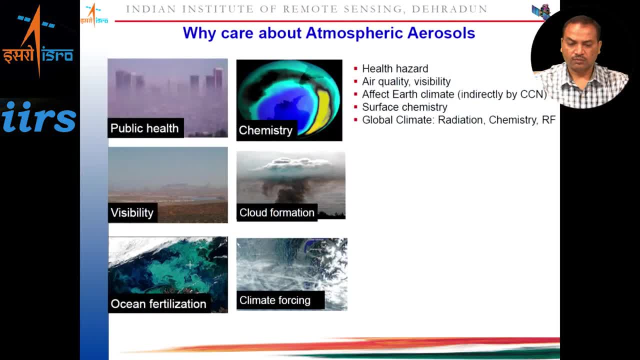 secondary sources of aerosols. now, why do we care about the aerosols? because these had a wide variety of the effects over the atmosphere, the ocean, the, the human dimensions and the health issues, and so the the number one is your health effects, health hazards because of the pollution. 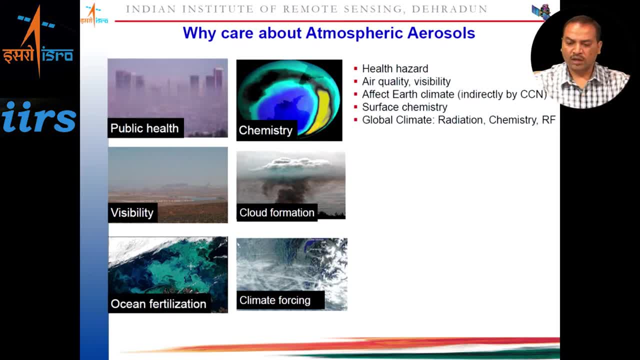 the, the health on the humans and the air quality, the visibility and the effect, of course, the effect of on the earth climate, because these, these also become as formed as a seed for the cloud condensation nuclei. so the, they, they also help in the formation of lot of clouds and which 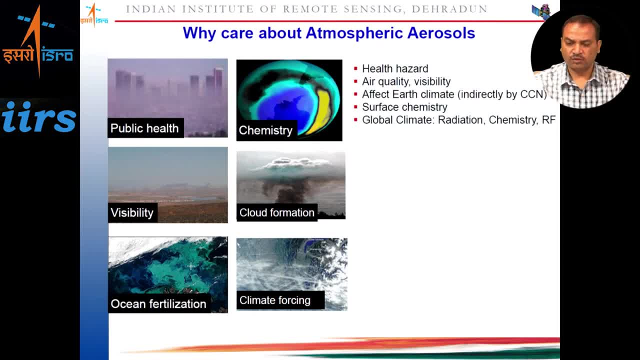 indirectly affects of more scattering of the sunlight back to the atmosphere and less amount of sunlight reaching on the earth surface and that is the dimming of the, the solar radiations, and which is a cooling effect over this and it affects the. all the processes, the biological and physical processes over the earth surface, of course, the surface chemistry. 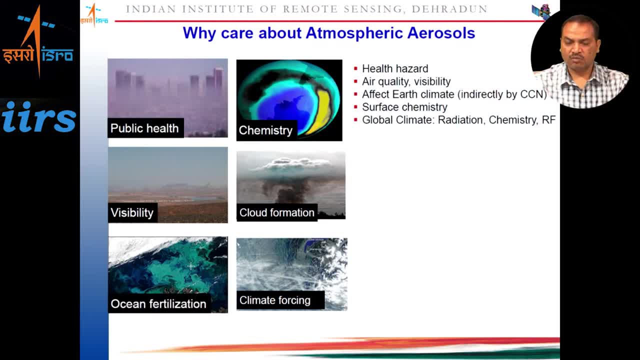 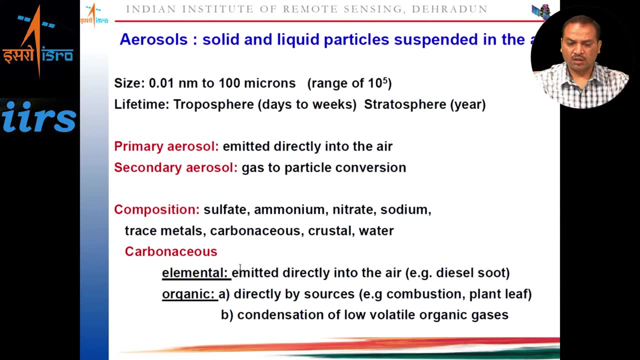 and the and the, as i said, the radiation budget and the chemistry and the change in the radiation flux, that is, the uh, the relative forcing, though it affects also the relativity forcing. so, as i said, the aerosols are solid and liquid particles, uh, suspended in air, so they are the. 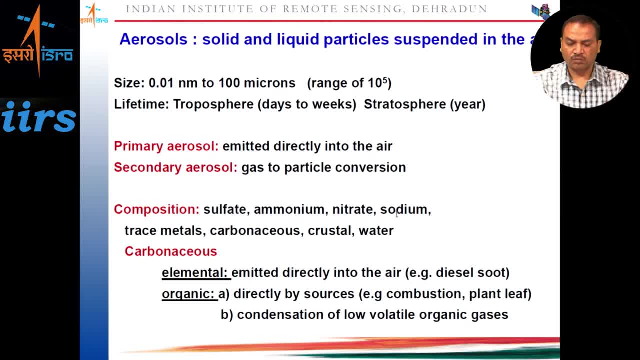 composition can be sulfate, ammonium nitrate and sodium, see the. the sulfate and nitrite contributes around three phases of oceanmarine addition of this neo energy and other elements of thisual jesteśmy and three-fourth of all, the composition of the types of aerosols. because and the rest? 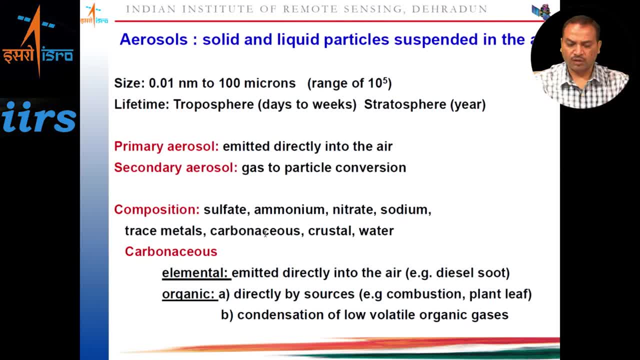 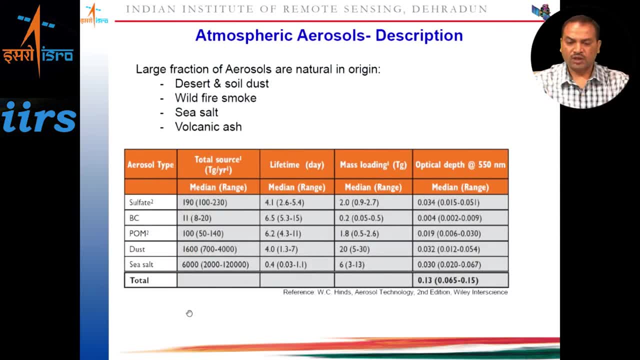 are your anthropogenic. anthropogenic consist of your carbonate aerosols, and these are elemental, and your organic. If you see about the dimensions of your the sources, this table, a glimpse of this table, shows that the most of the aerosols are sulphate, the particulate organic matter, the dust and 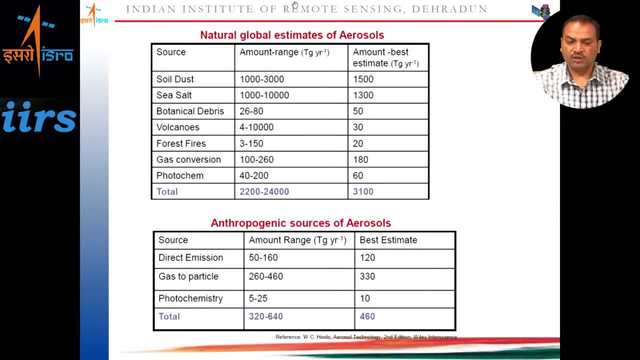 the sea salt and if you see your natural estimates of aerosol worldwide global average distribution and your the anthropogenic sources distribution, The main point comes here is about 85 percent of your aerosols are from natural, natural processes. 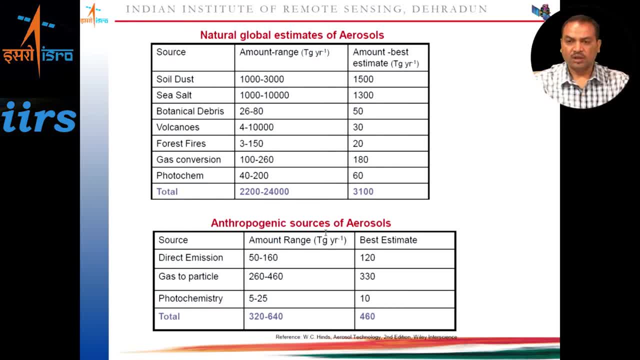 and your 15 percent is through the anthropogenic. The number may be small, but the effect of these aerosols from the anthropogenic sources is large, is huge and the over the decades and over the years the contribution of the anthropogenic sources are increasing tremendously. 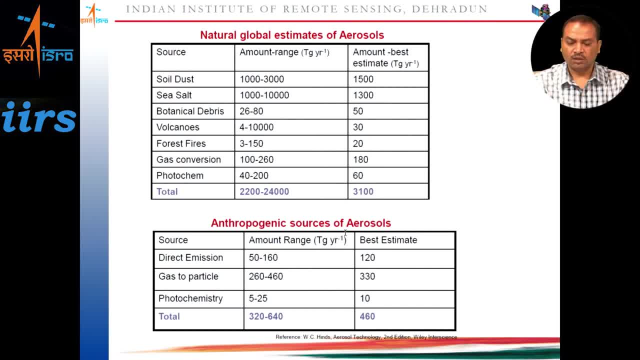 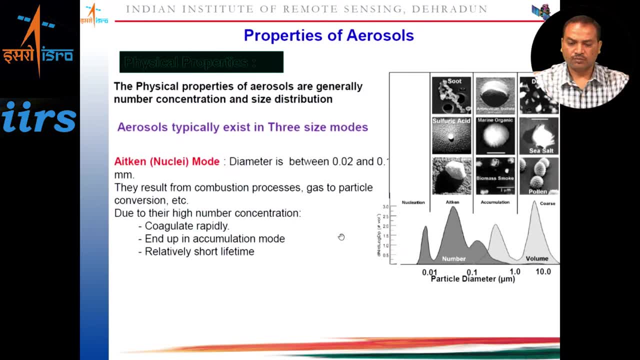 And the effect is huge over the ah, when we talk about the direct emissions, or the, your photochemistry, or the secondary emissions of from the anthropogenic. Now, when we talk about the ah, the properties of aerosol, ah, they are. they are the distinguish from the physical properties, the optical 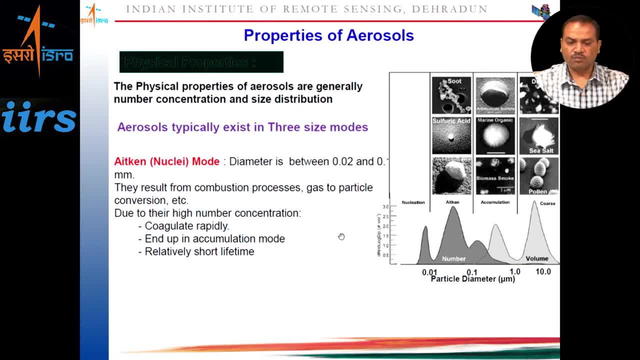 properties and the relative properties. So in terms of the physical properties, The consist of generally the number distribution, as I said, the number density, that is, in the one, in the particular volume of the air, how much number of aerosols exist, by number or by mass. So number distribution and the size distribution also. 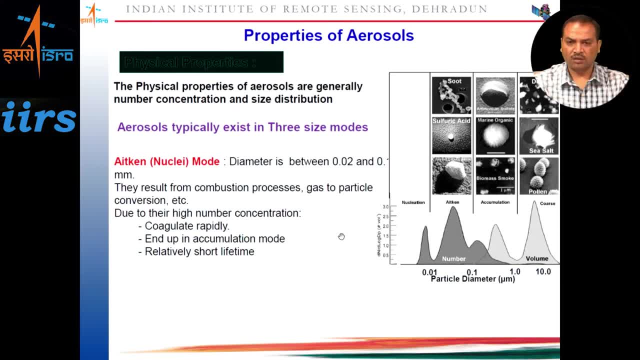 So what is the particle size, whether it is a fine particle or a medium particle or a coarser particle, because the the size also affects on the scattering and absorption issues of the light and it also affects on the number density also. The aerosol typically has three sizes. we divide into three sizes. we talk about Atkin mode, that is, diameter is 0.02 to 0.1 mm. 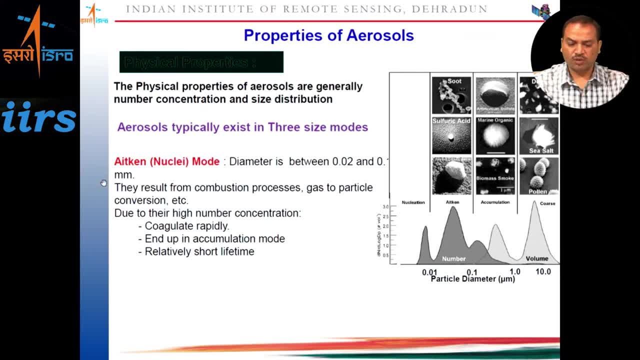 And the result from the combustion process from the air to the air, is 0.02 to 0.1 mm And the result from the gas to particle conversion and due to their high number- these are very high number, number density- So they coagulate together and then they form the next size particle, slightly bigger, larger, slightly bigger particle, which is known as the accumulation mode. 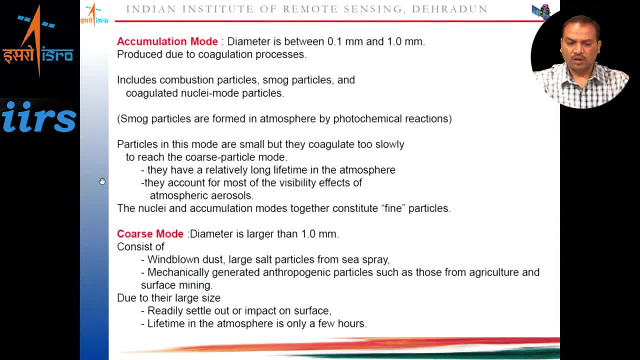 And the. the lifetime is very short and these Atkin particles coagulate in certain medium, the hydroscopic in nature, and then they form the accumulation mode. The diameter is 0.1 mm. This is between 0.1 to 1 mm. 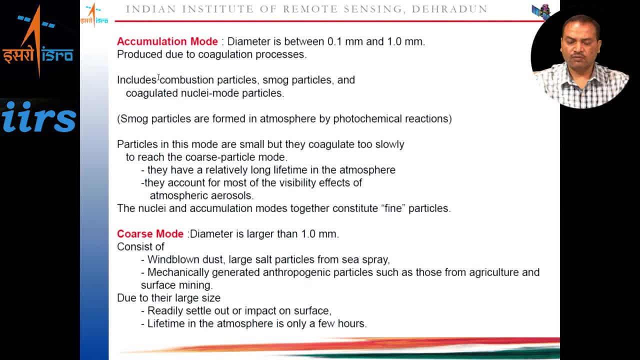 And this also includes the, the combustion of the processes of particles, the smog and the coagulated of the Atkin particles. More slightly larger particles, which are known as the diameter, the coarser particle or giant mode, or the particles having more than 1 mm size. 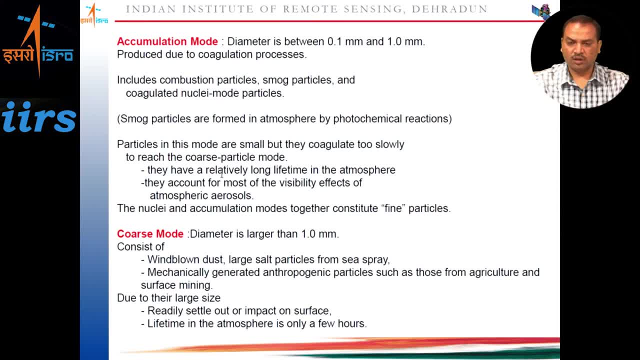 They consider the sources are from the windblown dust, uh, the, the sea salt particles, uh, and the mechanically generated anthropogenic particles from the agriculture or the mining activities. and due to their larger size, they settle down due to the gravity, because larger size or gravity, and then the lifetime is very. 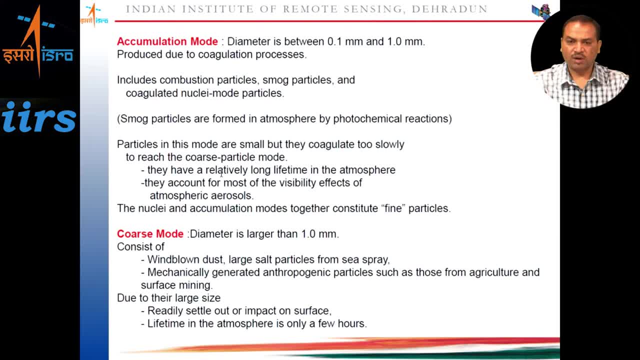 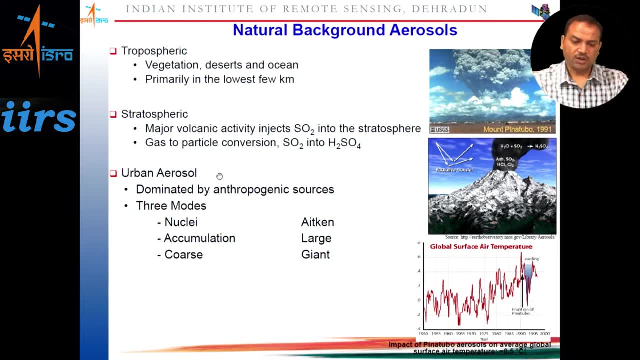 very low, maybe a few hours, so more. the larger the particles, the lifetime decreases. now, uh, the the natural background. when we talk about this, the tropospheric. the tropospheric are your vegetation, deserts and oceans. and when we talk about the stratosphere, because what happens is the aerosol particles greater than one micron size. 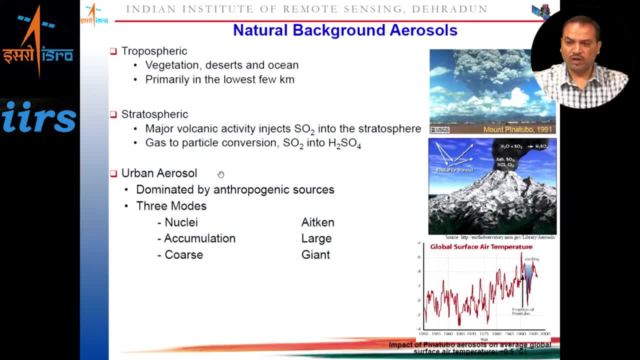 they are mostly produced by the windblown and sea salt and the particles, also the volcanoes, which majorly injects the sulfur dioxide in the in the atmosphere, goes in the upper layer state from the in the stratosphere and due to the process of the gas. 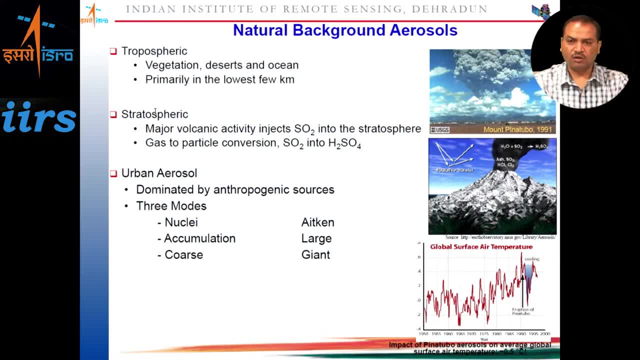 to particle conversion and the, the mixing of the, the sulfur dioxide, with the water vapor, it forms the, the sulfuric acid s2so4, and then the aerosols are transmitted and they mixed and transmitted by the atmospheric motions, uh, and they are removed, primarily removed by the clouds. 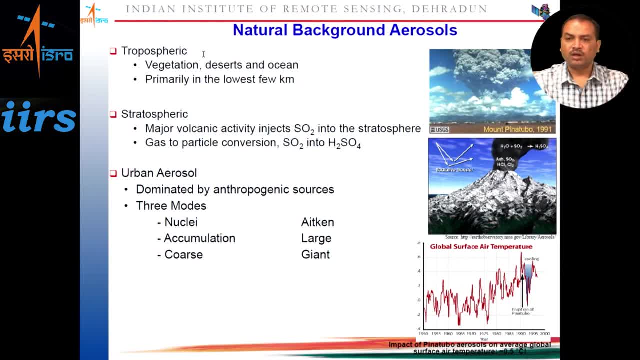 and the precipitation and they come back to the uh, the or the land uh. but these uh, the sulfur dioxide and they all uh are very effective in the uh transporting from one region to another region- very large region, they transport from large regions and the surface they are also transported from. 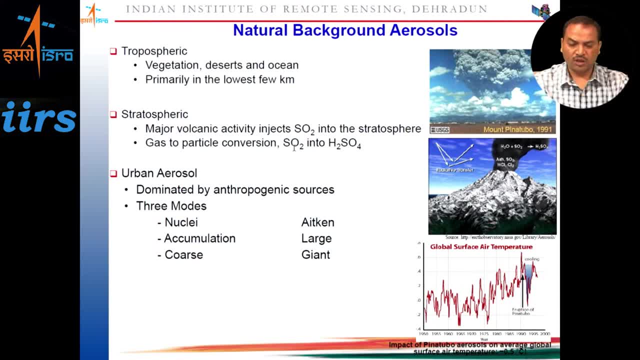 larger regions and they are transported from larger regions because these are very effective in the region and they form the clouds, and then they are responsible to prevent the energy reaching on the ground, and thereby they are also responsible for the global cooling effect. The amount of the cooling depends on the force of eruption of these types of volcanoes and 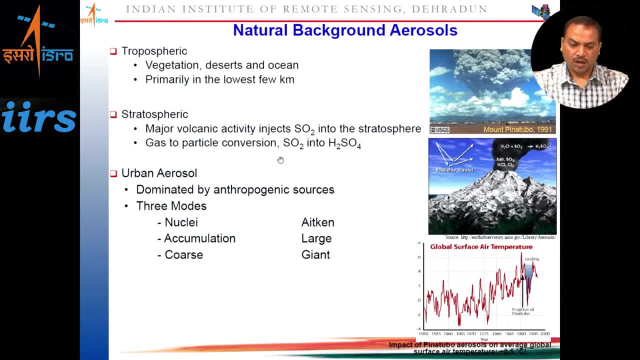 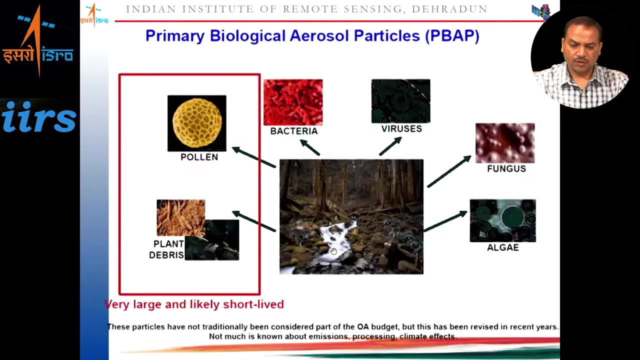 also on the on the prevailing wind patterns. In terms of the urban type of aerosol, which I said the sources in my previous slides. they are fine particles less than 1 micron of size, which is classified in three modes. So basically, basically here, if you see, 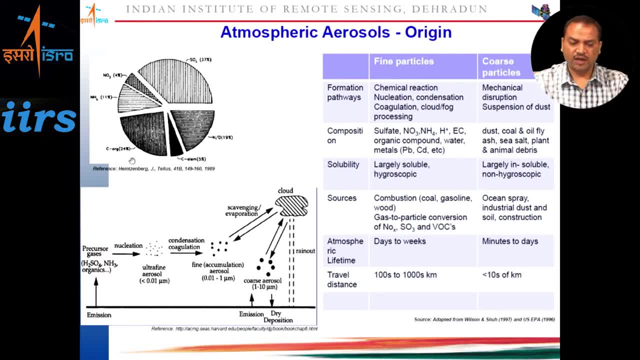 As I said, the, the sulphate and your nitrite consist of the three-fourth of the these particle types, and these, these are also responsible for the, the formation of the different types of aerosols. Now, when we talk about the composition of the sulphate particles, these are, as I said, 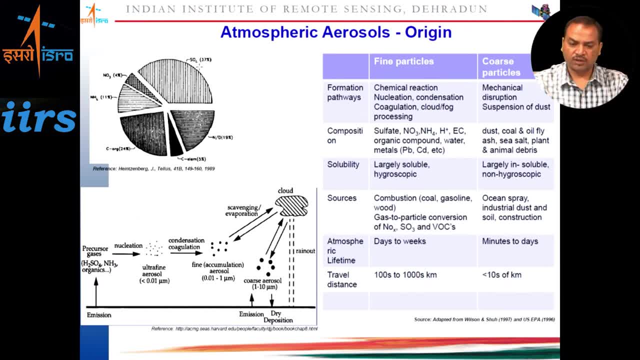 the. these are modified by the sulphur dioxide and the water vapor combinations, and then the organic carbon, which is around 24 percent, The it. it represents the, the fraction of the fine aerosols, the and the condensation of the large hydrocarbons of biogenic and or the anthropogenic origin. ah, and also, if you. 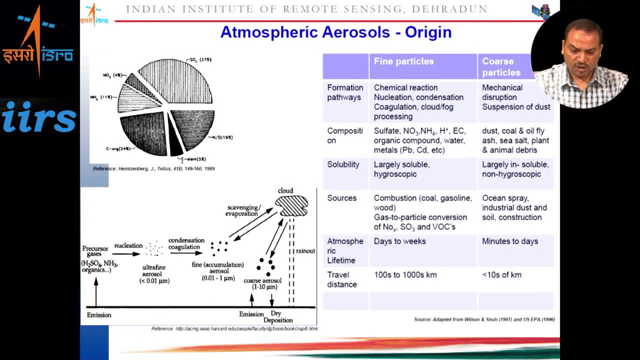 see the elemental carbon, the anthropogenic soot particle. This is produced by the condensation of gas during the composition and is it is commonly, as I said, it is, known as the elemental carbon or the black organic aggregates of the compounds. Now this figure shows the production, the emission, the sources. 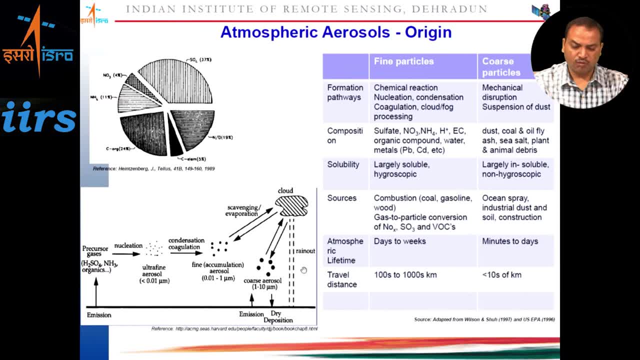 the production and the growth and eventually the removal from the atmosphere of the aerosol particles. Now, the gas molecules are typically, as I said, it is very low in number, very small in number and the sizes are very, very small. They coagulate, they cluster the sub, the 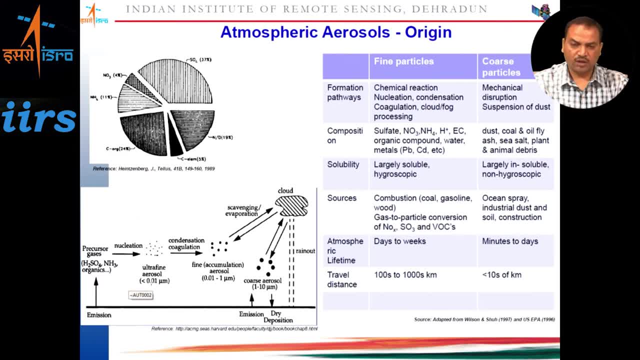 ultrafine, the aerosol, which are less than 0.01 micron in size, And these are the precursor gases which I said, the sulfate and nitrites, which constitute three-fourth of the particle types, and these are very small in number, less than 0.01 micron. 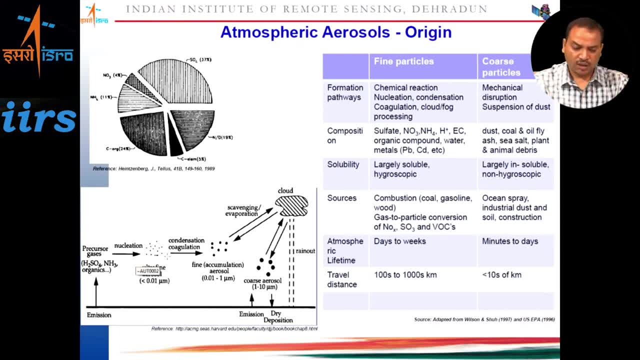 ultrafine and then they coagulate together and form the accumulation mode, which is 0.01 to 1 micron. and these again when they coagulate, because coagulate, because the collision between the particles during the random motion, and then they coagulate. 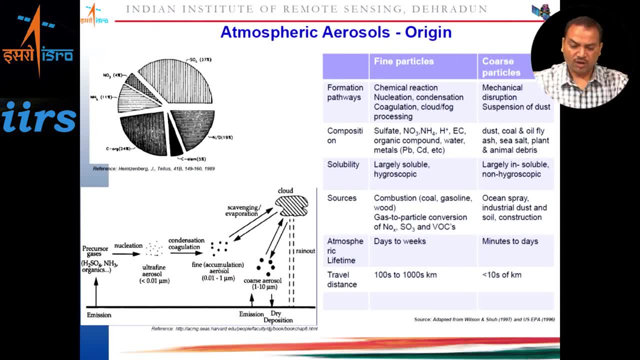 And they form the accumulation part of types of particle. Now these particles are too small to sediment at a significant rate and are removed by the atmosphere mainly by scanning, by the cloud droplets and the scanning, and also by the evaporation and forming to the 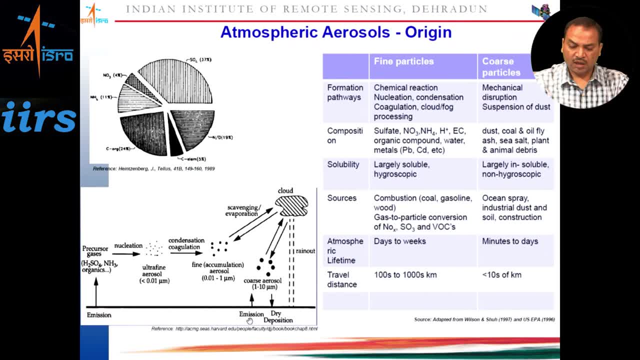 clouds Again, the there are again sources for the coarser particle. as I said, the wind blown, sea salt spray over the ocean and the over the land. they are responsible for the coarser particles around less than 10 microns and they also, as i said, due to the large size they settle. 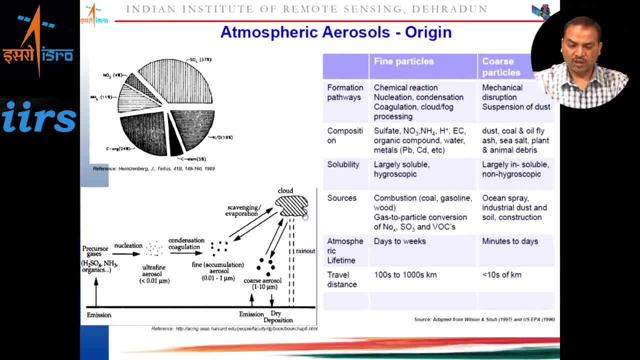 due to the gravity and by also the washout by the rainfall. so they also having either the dried deposition due to the gravity, as i said, or due to the wet deposition due to the washout by rain, and also these particles, when they are in the atmosphere, they also responsible for the cloud. 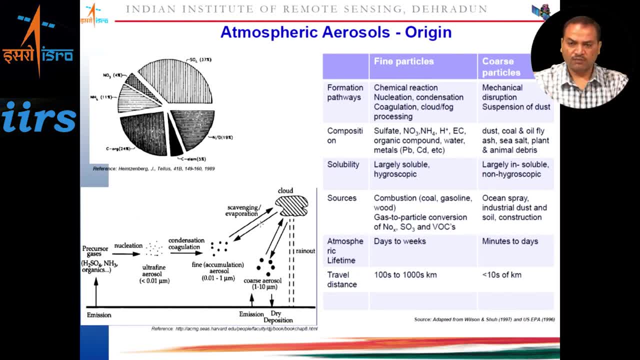 condensation nuclei for the they form as a seed for formation of the clouds and then they have an, a combined effect. they have a direct effect- direct scattering, absorption- or a indirect effect wherein they form lot of clouds and affecting your surface albedo, or or the albedo of the clouds. 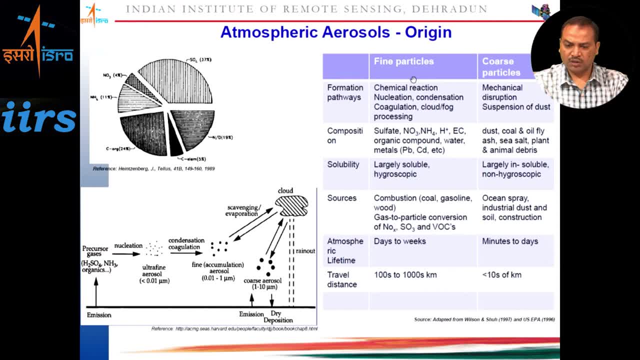 this table gives you a feel, the of the fine or the coarser particles, in terms of their, the formation, that is, the, as i said, is written here, the chemical reactions, nuclei, as i said, the coagulation and the cloud and etc. and the, the coarser particles are the disruption, that is the. 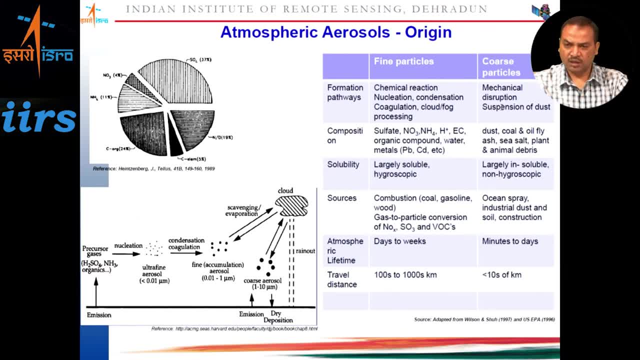 mechanical, distributed by the wind blown dust. the composition: as i said, the sulphate nitrates and more of the particles are distributed by the wind blown dust. ammonium and same nitrates, the elemental carbon compounds and the coarser particles are your dust, the sea salt and the the practices over the land and ocean. in terms of the solubility of these, 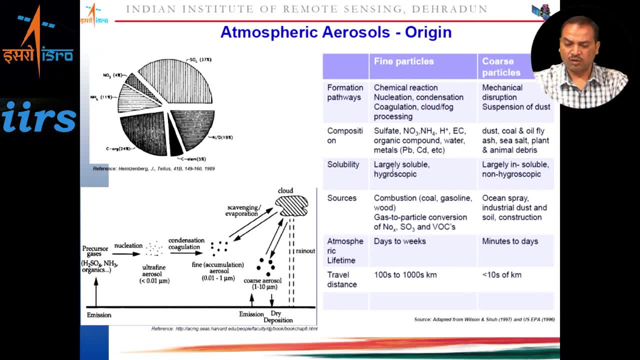 types of particles. the fine particles are largely soluble, that is, hygroscopic in nature, and the coarser particles are largely insoluble, that is, non-hygroscopic in nature. uh, the same. the sources are now given to you: the, as i said, atmospheric lifetime. the coarser particles are having less lifetime as compared to a to the fine mode particles. 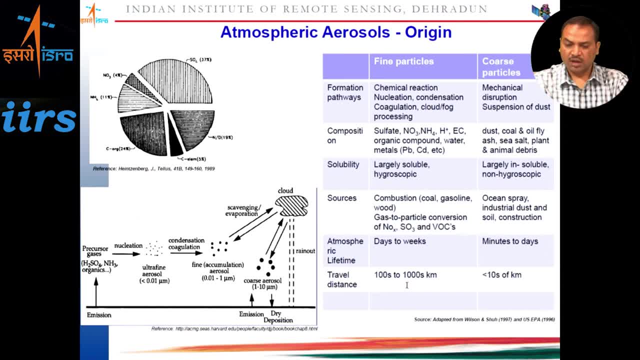 and the very important aspect is the distance. they travel the coarser particle: due to the larger size and the gravity settlement, they don't travel much, maybe few tens of kilometers. but the fine particles, they are a regional or continental particles and they travel through hundreds of thousands of kilometers from one region to other region, depending on the environment. 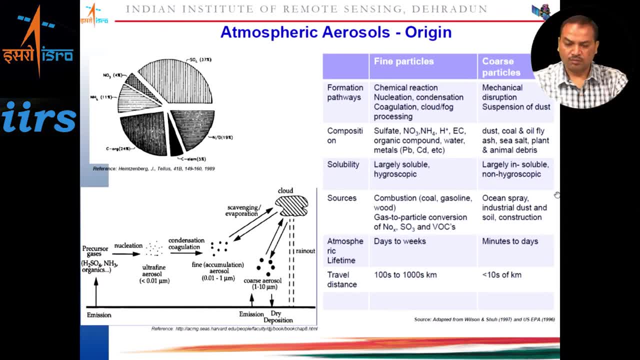 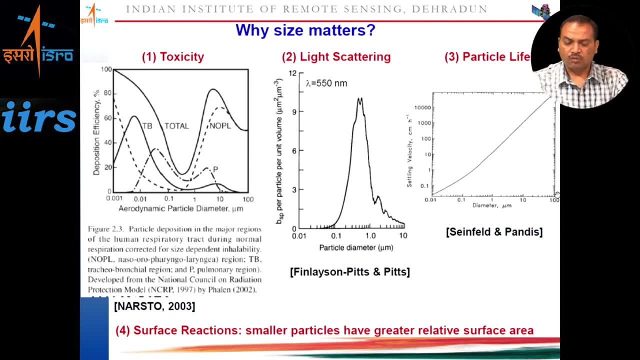 and the and the wind motion vectors, how they follow them. now, why is so important about the size of the aerosols? now, because the i try to classify into four categories: the toxic of the nature, because, as i said, it is also impacting your health. hazard, uh, and in this graph you can see that. 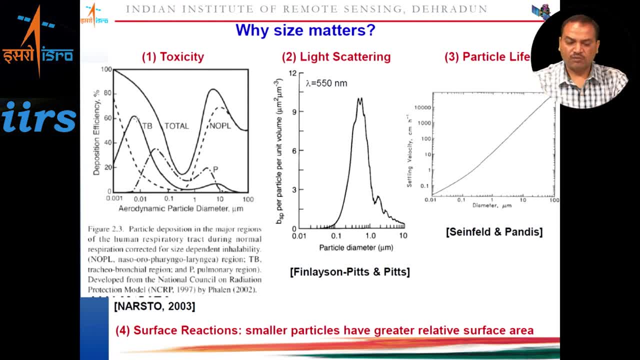 this graph shows that is the responsible when we inhale these particles. we are very small in size, so these are easily inhalable by the humans and the, the bronchitis or the muscular, which are where it deposit. very important- the passage from the nose to the lungs, and there are many. 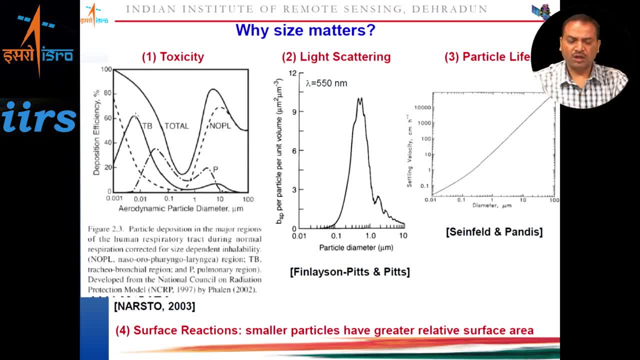 areas and they travel through the, the cardio and the respiratory muscles. if you see the graph, a total graph, the more is the fine particles, the finer particles, the the deposition efficiency is high. if you see here the deficiency, the efficiency is high. so the more it deposit, so it becomes an toxic in nature and then it affects your health. 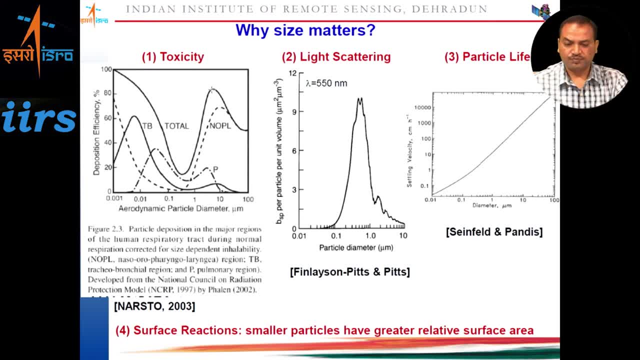 the more of the fine particles. the health issues are more in terms of the light scattering, the. as you know from the law of physics, the rayless scattering, or the b scattering, the. the scattering efficiency increases when the particle size is equal to the wavelength, so the, the one one less than one micron. 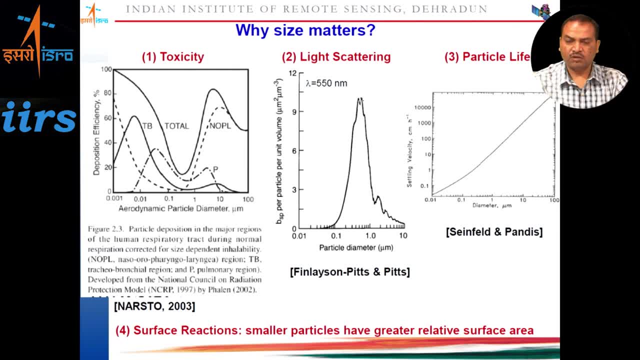 the particles, the efficiency is very high. that is the. your scattering efficiency is very high, that is the particles less than one microns and if you see the particle lifetime, the y-axis shows you are settling velocity. so more is the your particle size. the settling velocity is high. 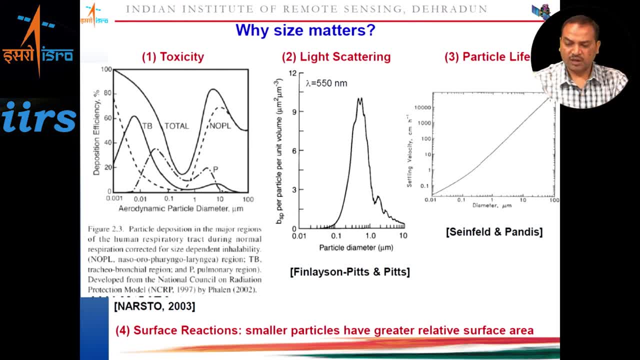 so it means the: as the particle size increases, larger particles, they settle more easily and their lifetime is less, so as the fine particles, the lifetime will be more. and if you see the reactions, the surface reactions, smaller particles have greater relative surface area so they react much, leading to the secondary or the, the photochemistry in the photochemical reactions in the atmosphere. so 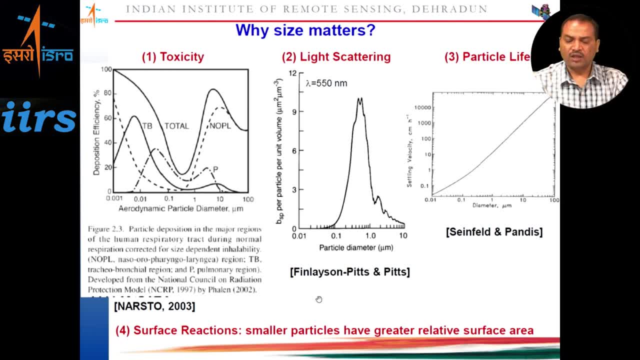 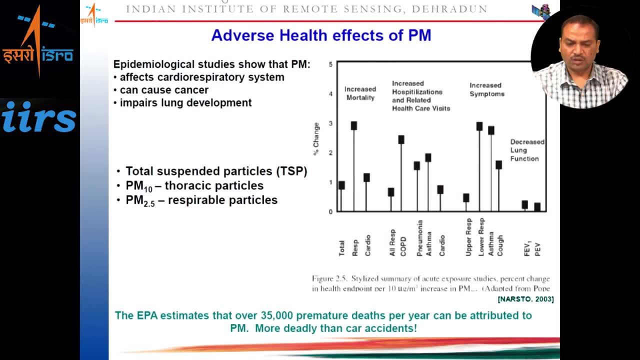 So the problem with the and the effect of the finer particles is more as compared to the coarser particles. Now, this is the same slide which I said, that particle, now the particle size, the total suspended particles are divided into 2, 3 categories, like the particulate matter, the aerosol particle. 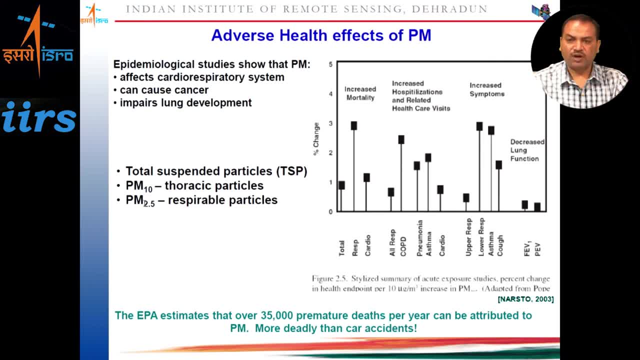 matter less than that is all the particles less than 2.5 microns are deposit and terms, as PM 2.5 and PM 10 determines the particle size is greater than 2.5 but less than 1 microns and this total addition is total suspended particles. 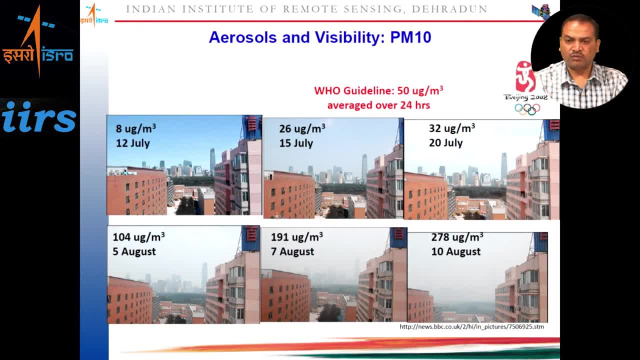 So there are certain guidelines which are in the atmosphere, air pollution studies. these guidelines are being used and you see now and then in the newspaper, on the media and the air quality index, the, which has been given for most of the cities, So the particle PM 2.5.. 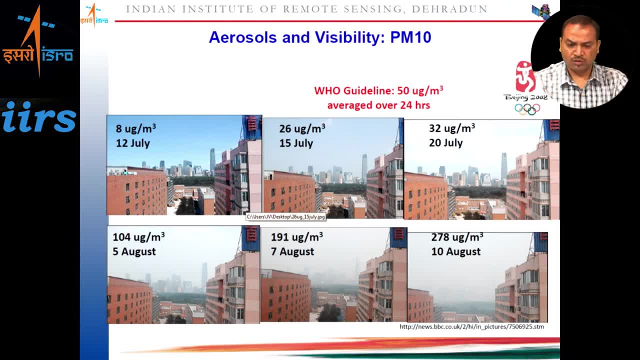 PM 2.5 is an important factor which is responsible for your air pollution. just a just a glimpse of this Beijing 2008. you see that in during the Olympics, the due to the pollution and other things, they try to maintain the air quality standards and the mainly the industrial. 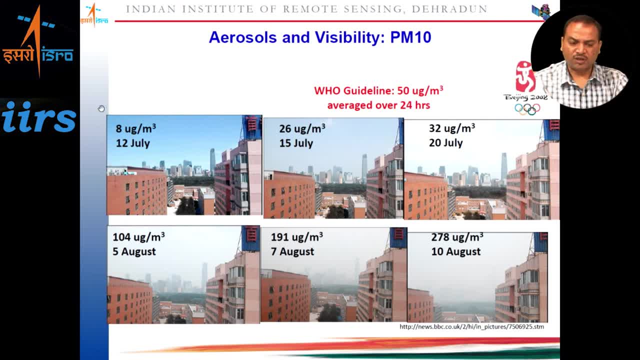 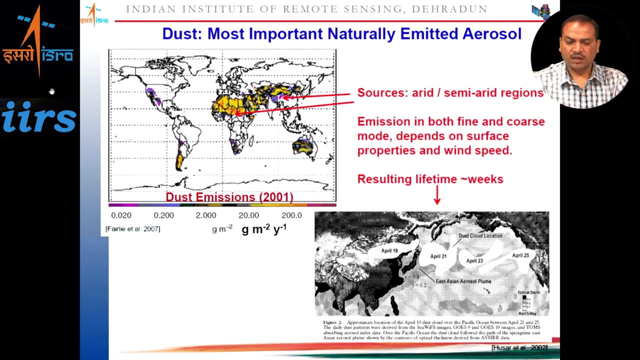 and the anthropogenic and they have taken all the cities. there is a vast problem in the to control the air pollution and the WHO guidelines are 50 micrograms per meter per cubic meter and that average over a day and this has to be maintained For a perfect the the air, air pollution in terms of the air pollution indices. 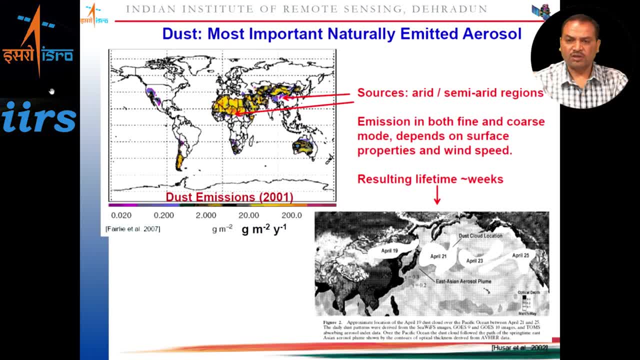 Now, as I said, the, the aerosols which are emitted, the transport from 1 region to other region, because they are not stagnant or station at one place, so the sources and the sinks can be different, Demeter most of the dust from the Sahara. they travel to the many continents and then it travels at a 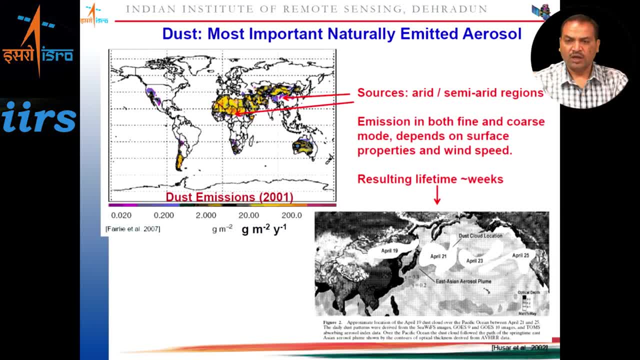 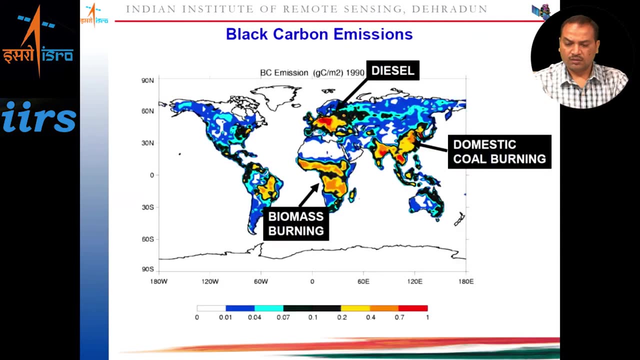 different layers of the in the atmosphere and then it has an effect over the, those region where it travels and one has to study the. one can study the, what is the concentration and where they are traveling from one place to other place and what is the lifetime In terms of the anthropogenic 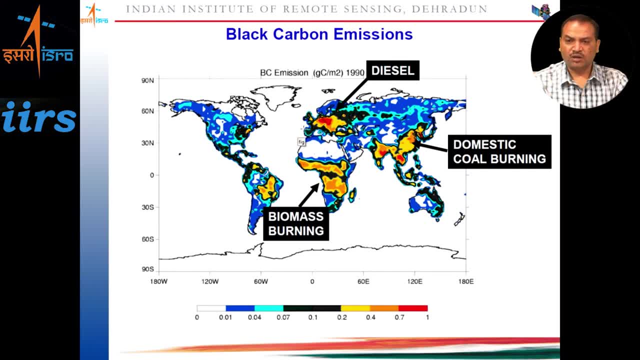 black carbon emissions, as I said, they do: the human anthropogenic emissions, either through the biomass burning or the fossil fuel burning, or the fossil fuel or the biomass burning, and different regions have different propositions. because if you say about the Europe, most of the emission of the black carbon is due to the biofuel, as compared to the Asia, which is mostly your. 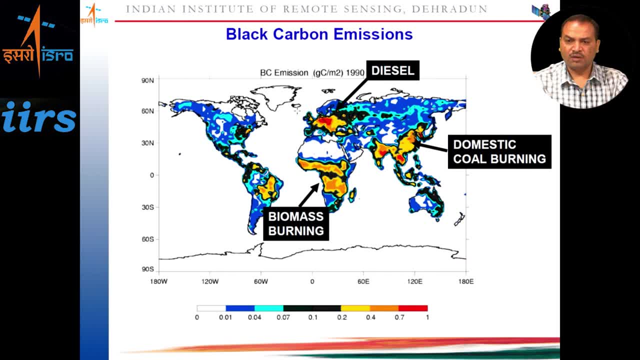 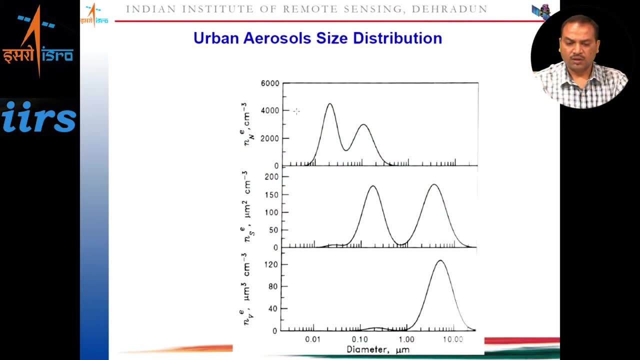 the, the, the, the, the domestic burning or the deep, or the biomass burning, biomass burning through the practices of the agriculture, residue burnings or the forest fires, etc. now, as i said that the, the fine mode particles are mode contributors, are from the anthropogenic emissions. now this clearly shows. 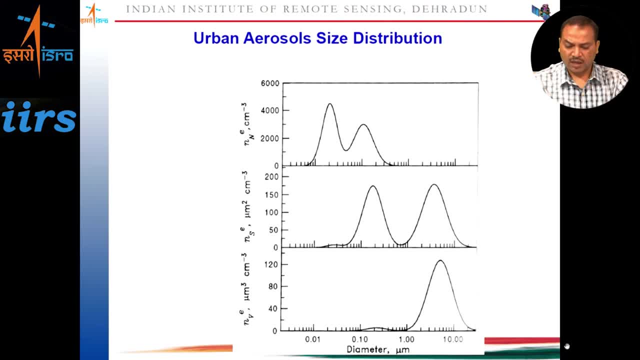 the y-axis shows the number density profile and the x-axis shows your the sizes of the particle. if you see the, the, the anthropogenic emissions, here is more. the number density is more because the fine, more particles are more here. so in the urban aerosol type size distribution. 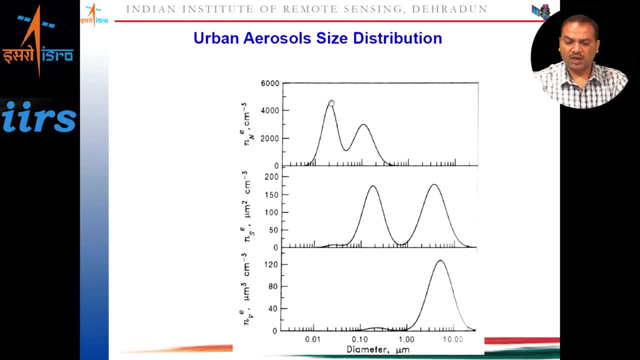 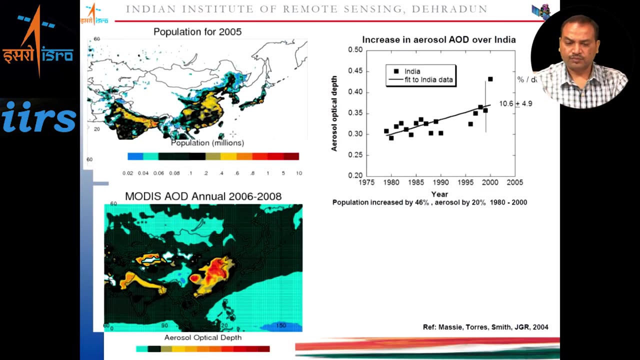 we find such type of distribution where large aerosol number distributions are are seen or are studied, uh over, the uh fine or the uh less low size particles or fine mode particles, if you talk about over india, as because more of the population, more will be the emission, because 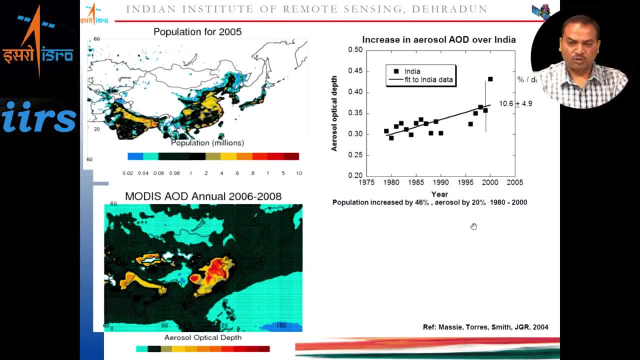 of the anthropogenic practices and anthropogenic activities. so this is directly relation with the population and the activities and if you see over the from 19 1970s, the, the emission of the aerosols- average aerosols are increasing over indian region and it. it is also applicable to 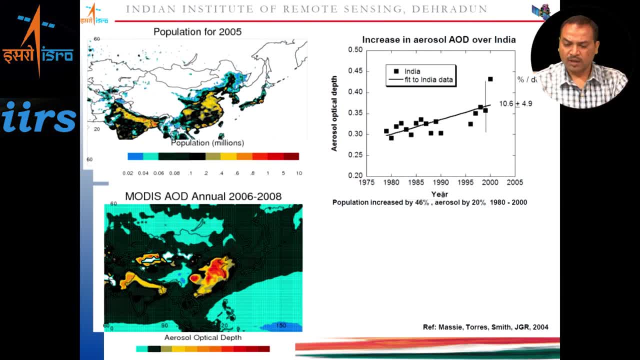 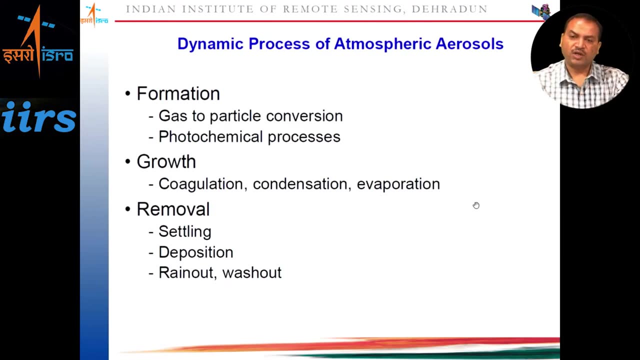 whole whole world where everywhere it is increasing and the population has increased over last three decades- three to four decades- around 46 percent and aerosol is around 20 percent. so 20 percent of, on an average, has increased. that is the. this directly shows the how the effect of the anthropogenic emissions are increasing from decade to decade. 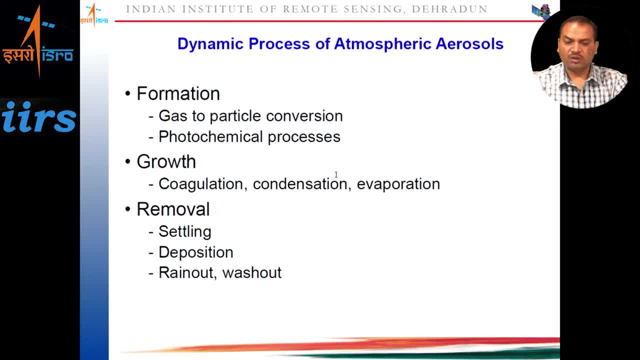 so the the dynamic process of the atmospheric aerosol can be summarized as follows: that is, the formation and the growth and the removal. in the formation, the gas to particle conversion, the gases animation and the particle and convert to the particle with the hygroscopic nature. then it also reacts with the in the atmosphere, which is known as photochemical processes. 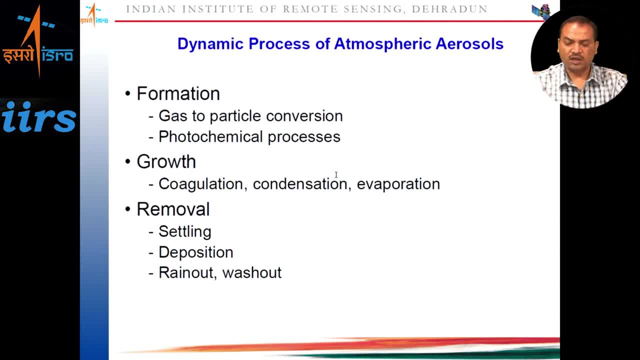 then also the fine particles coagulate, and the condense, and also the evaporate, and also they. they also acts as a seed for the cloud condensation nucleus, and then it, as far this removal process is concerned, it is settling down to the gravity, the dry deposition, and by the, the wet deposition due to the rain. so these are the cycle of the. 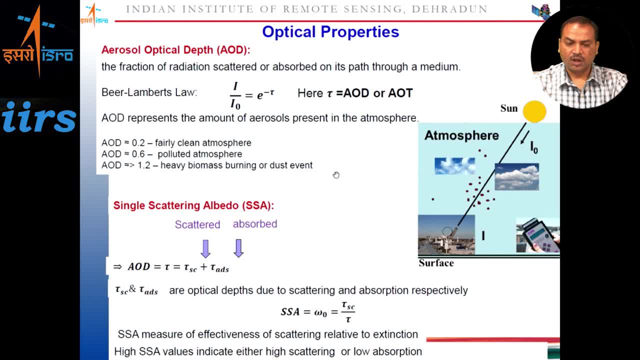 aerosol processes. now, as i said, one one property was the physical property. another property of the aerosol is known as the optical properties. the optical properties is the aerosol optical depth, so the, the, the fraction of the radiation scattered or absorbed on its path through a medium. 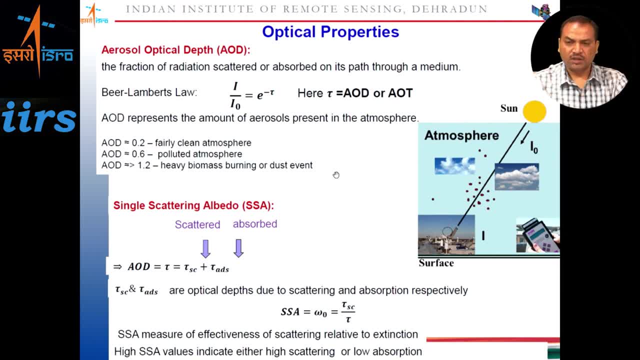 so whenever a light travels in the atmosphere, the how much it travels, that is, the length, the path length, and the the amount of fraction of the scattering or absorption it it handles or it enables during its motion. so there is a. this equation was given by the beers lambert and that 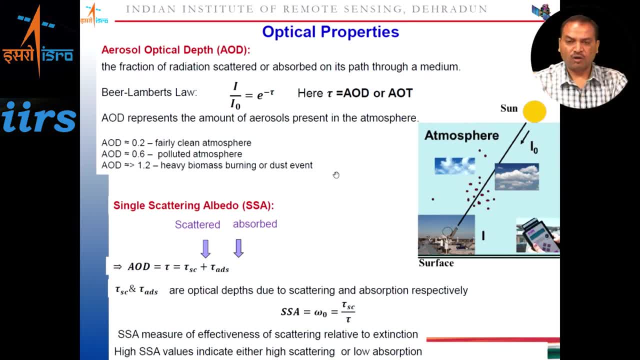 is, i is equal to. i naught into exponential of your one factor which is known as your, the aerosol optical depth. so this aerosol optical depth represents the amount of aerosol present in the atmosphere, indirectly, the what is the amount of hindrance given to the light traveling in the atmosphere? 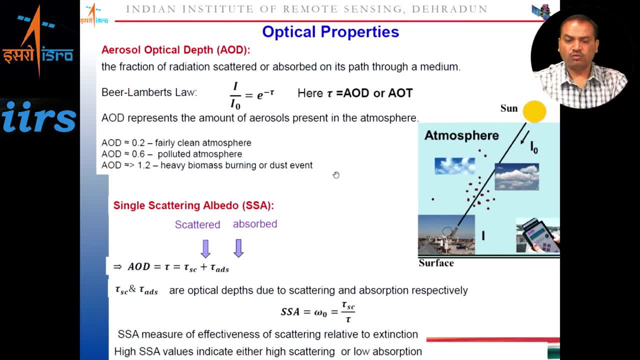 at a particular path length can also be indirectly be used to calculate the amount of the aerosol present in the atmosphere. so this equation can be indirectly inverted and the tau, which is known as the atmospheric aerosol optical depth, can also be estimated on the amount of the atmosphere, and it is a unitless quantity between 0 to 1, being 0 is a. 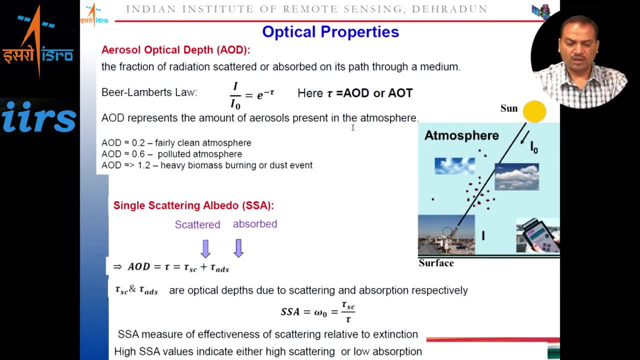 cleaner atmosphere. that is, less amount of aerosol, and 1 is the maximum amount of aerosols. and when there is a huge dust, episodes, huge dust, then the value can also exceed more than 1.. Another optical property is a single scattering albedo. the single scattering albedo is the measure 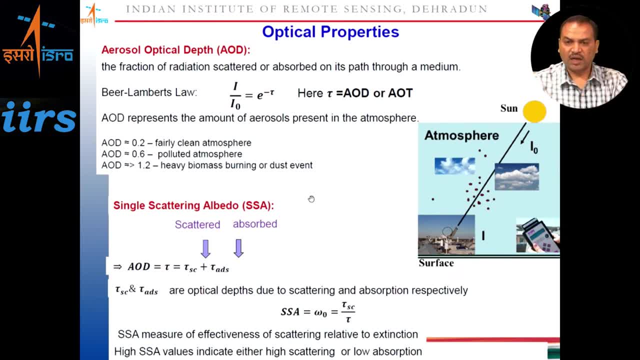 of the effectiveness, how a particle can scatter relative to its absorption. So whether now we know that the amount of aerosols are there, but we are not aware of what are the type, what is the quality of the atmosphere, whether it is a scattering type of aerosol or whether it is. 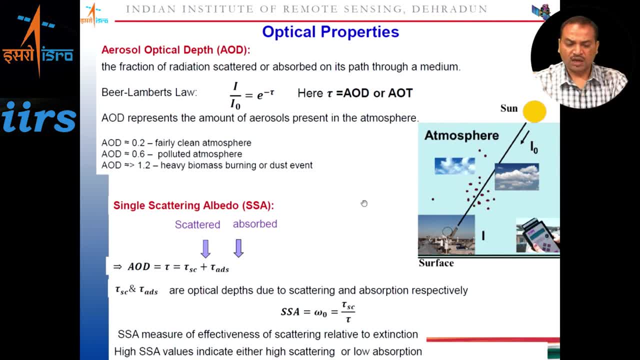 a absorbing type of aerosol. So the single scattering albedo gives a picture or gives a indication of the type of the aerosol, whether it is scattering or whether it is a absorption. So the ratio of the scattering to the total extension, Extension means it is the combination of your total scattering and 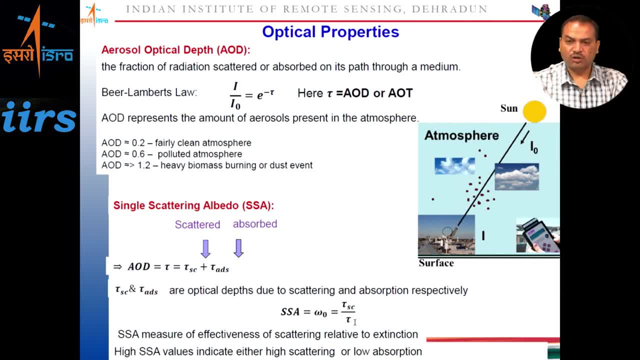 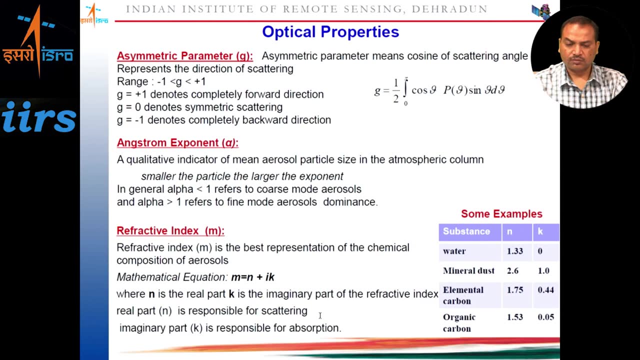 absorption- So it is a value- is between 0 to 1.. So 0 means total scattering sort of absorption and 1 the high value. sorry, the low value relates to the absorption and high value relates to the scattering. and another optical property is a asymmetric parameter, meaning to the cosine of the scattering angle, the 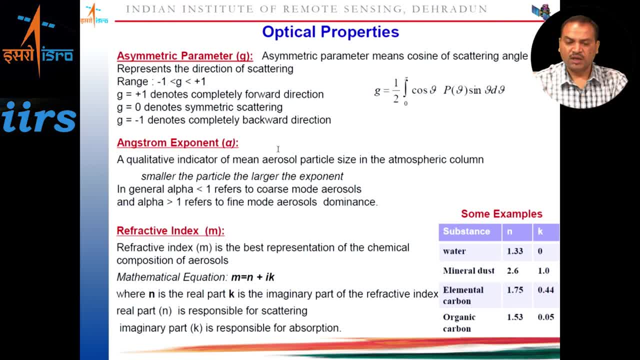 it is. it is denote 0 minus 1 and plus 1. it means that if the scattering is happening, the where is the direction of it. So this gives a relative direction of the of the scattering, The plus plus the signature. the sign symbolizes the forward direction and minus symbolizes. 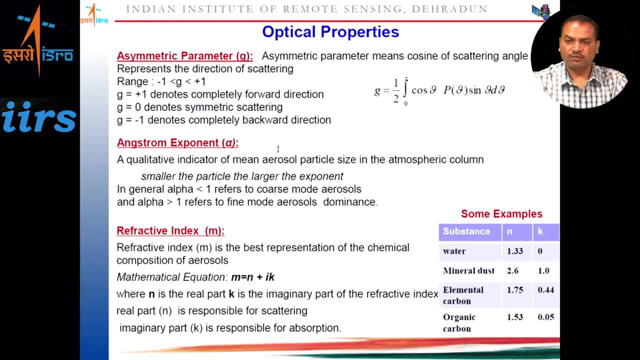 the, your backward direction, and 0 is a symmetric type of scattering. The angstrom exponent, another indicator of optical properties, gives an indication of your mean aerosol particle sizes. The physical physical sizes can be measured, as I said, from the previous slide, the physical properties, but also from the optical properties. one can 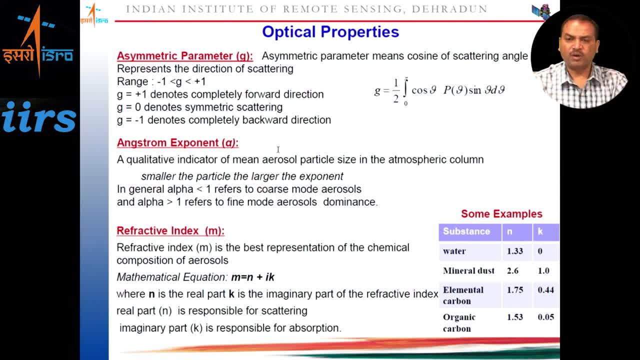 gain a glimpse of or indicator of the type of the aerosol particles, A picture of the aerosol, how, whether it is a fine mode particles or a coarser mode particles or a combination of both these type of particles. So the the less is the value of your the angstrom exponent. it means 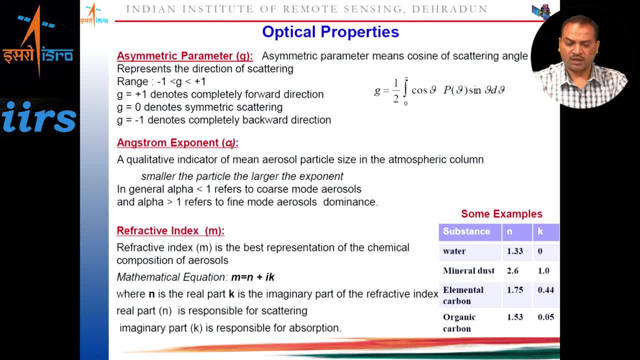 the particle size are a larger, larger size particle, that is, coarser particles and the high value denotes your fine mode particles. The refractive index and the ah, the. the refractive index is best representation of the chemical composition of aerosol. No, mathematically, when we see, we have learnt. 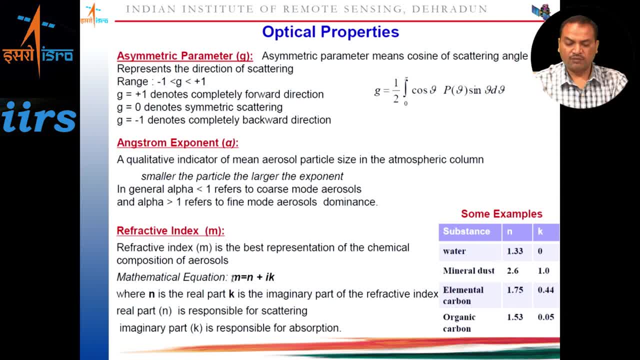 in the our school days that the ah, the refractive index, as in a real part and an imagery part, as I mentioned here, m is equal to n plus i into k. So n is your real part and k is your imagery part of the refractive index. Now, ah, here are some examples. if you see the water, 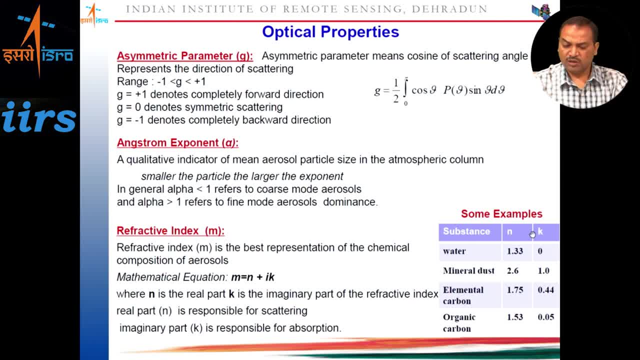 mineral dust, elemental carbon andocautic- Here the water does- and fashioned so at certain organic carbon: the real and imagery part. from the indication of the real imagery part we can estimate whether this type of particle is a scattering nature or a absorption nature. so 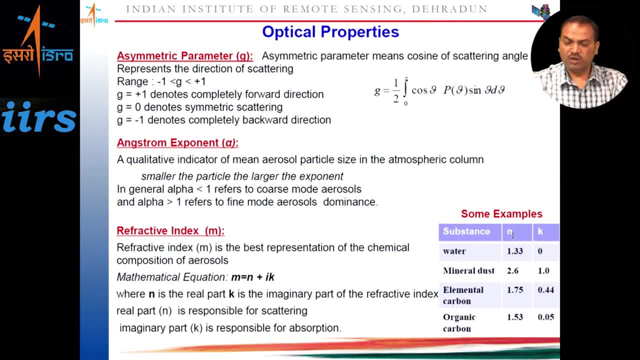 the more is your real part, the more it means, the more the number or more the value of this. the real part means the particle nature is scattering in nature. for example, water 1.33 and 0. mineral, for example the organic carbon 1.53 and 0.05. these are scattering in nature. and if 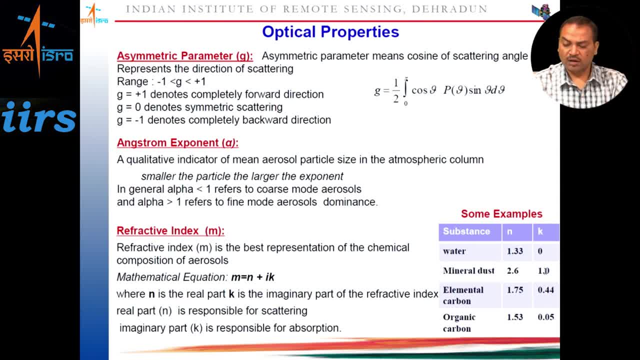 you see the mineral dust. it is 2.6 and 1. it means the more is the scattering in nature, but also it has a substantial amount of absorption. so here the problem is that sometimes the mineral can behave in a form, the scattering, and also in a absorption. so it has a good, good characteristics. 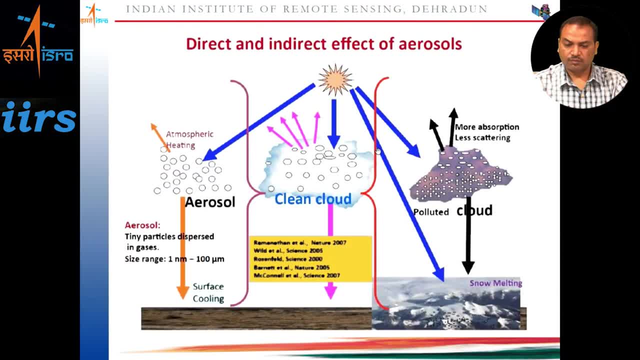 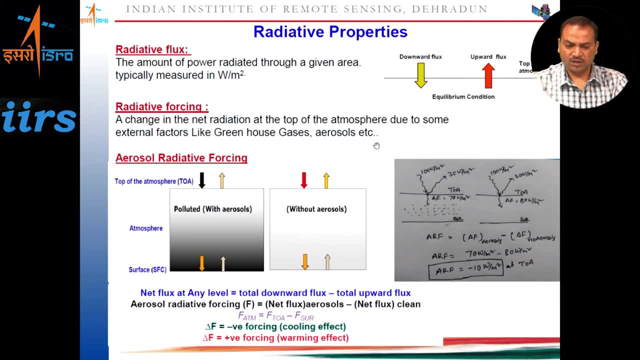 of absorption. also, the third, broader category of properties is the radiative properties, which is the, as i said, the. if there is a, if there are no aerosol, that cleaner atmosphere it means there is no hindrance given it and the amount of solar radiation, what it reaches at the top of the atmosphere. 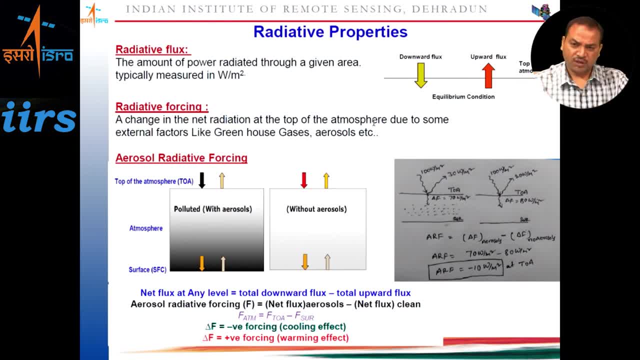 also reaches at the surface of the surface of the earth. so there will be you equal amount. there will be no change in the solar flux leaching on the surface of the earth. but if there are some constituents, particle, constituent particles, for example aerosols- they try to absorb or scatter and try to reduce or increase in the the sunlight reaching on the 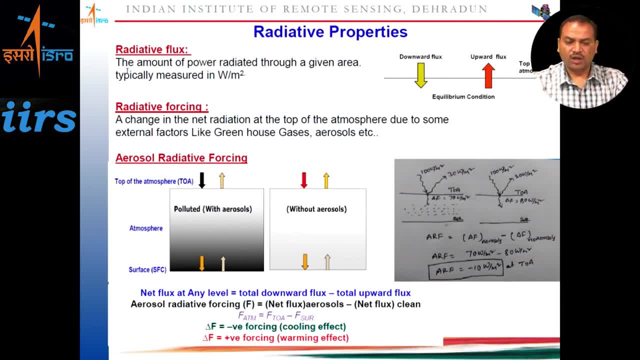 earth surface. so this change is known as the change in the net radiation at the top of the atmosphere and at the surface is known as the radiative forcing and the, the, the. the culprits may be anything, maybe the trace gases, the greenhouse gases or the aerosol. so we 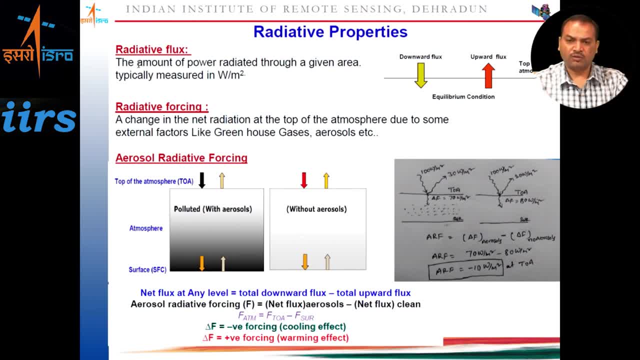 can say the relative forcing due to the aerosols and then the trees gases, the greenhouse gases, meaning the effect of the greenhouse gases on the relative forcing. so that's why we differentiate and we have abbreviate with our relative forcing. now here the datas. you have this Fourier directed force, which we call the passive force, receiving the loss gasiff in order for haters acá. 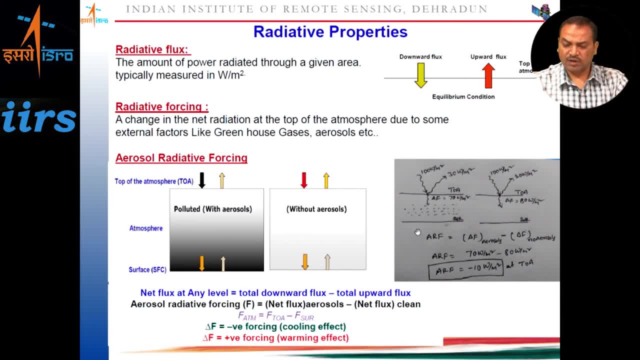 Now here the example is given here. for example, 100 watts per meter square of the solar radiation is reaching at the top of the atmosphere and the normal, the reflection, the 30 percent, the albedo reflection from, so the net amount of the relative flux which are reaching at 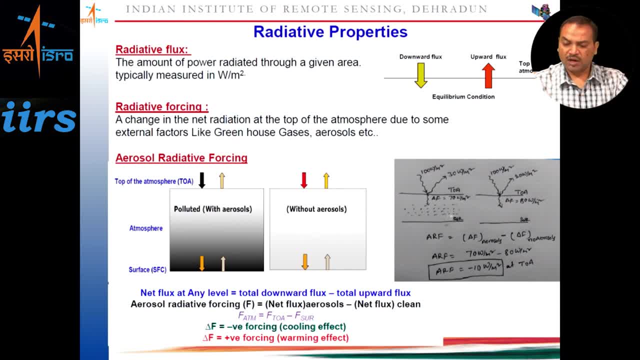 the top of the atmosphere is 70 watts per meter square. Similarly so, and in the first figure suppose there are aerosols here there are aerosols, So the amount of reflection is happening more, So that is 30. So it becomes 70 watts per meter square, and if there is no aerosols the reflection may. 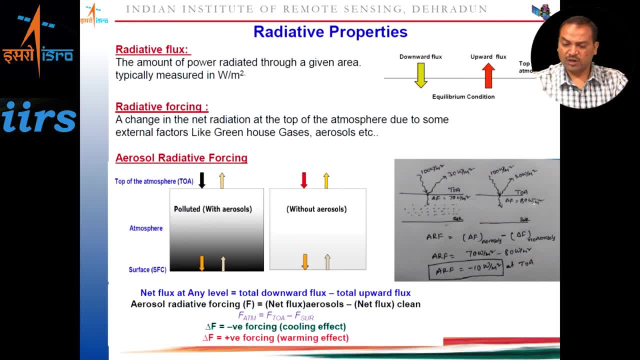 be less the 20. So it becomes 80 watts per meter square. and when you calculate the relative forcing, So it becomes a relative forcing is: and the net radiation net flux due to the aerosol, minus the net flux without aerosols. 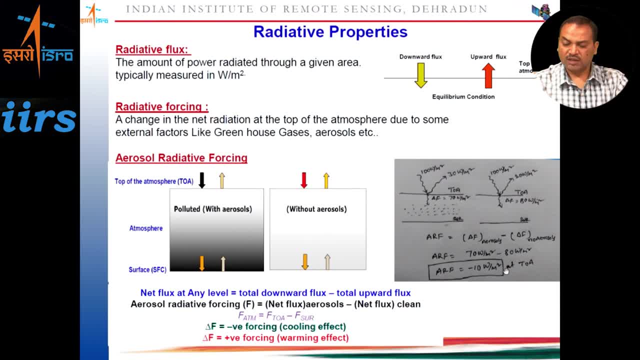 So that is 70 minus 80. So it becomes minus 10 watts per meter square. it means there is a cooling in nature, So less some. that is the due to the aerosols. there is a net cooling at the top of the atmosphere. 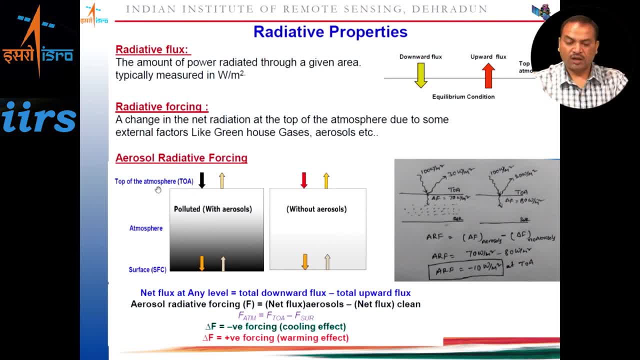 So similarly we can calculate the, the relative forcing at the top of the atmosphere, Relative forcing at the surface of the earth and also the relative forcing in the atmosphere. So the balance of these two, top of the atmosphere and the surface, gives they the balance of. 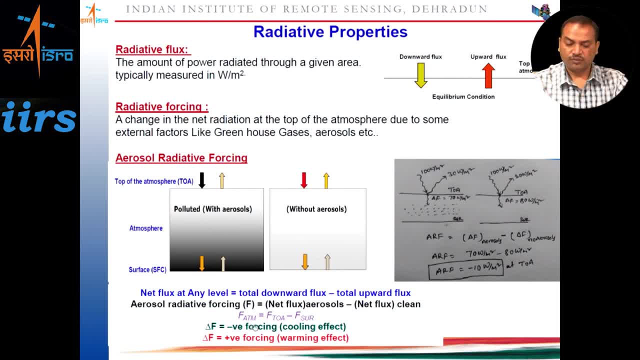 the relative forcing what is happening in the atmosphere. So this, the relative forcing at the atmosphere, is equal to the relative forcing top of the atmosphere minus the surface. So we can also calculate that whether the aerosols are heating the that is the more providing more flux to the atmosphere. 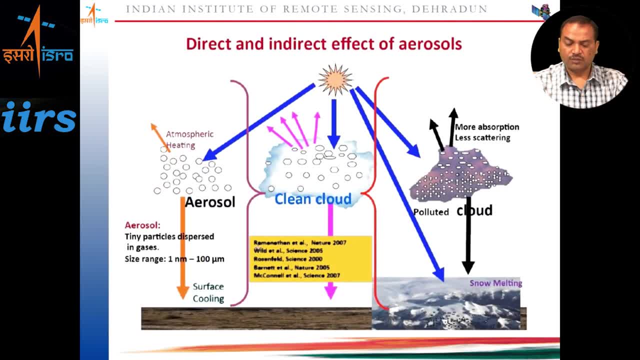 or is cooling. Now, broadly, the effect of the aerosol can be classified: direct effect, which is that is directly scattering and absorption the sunlight, and also the indirect effect. indirect effect meaning that the they, they are modifying the amount of the micro physical and the rate of properties of the cloud, that is, the cloud condensation nuclei, and with the limited amount, 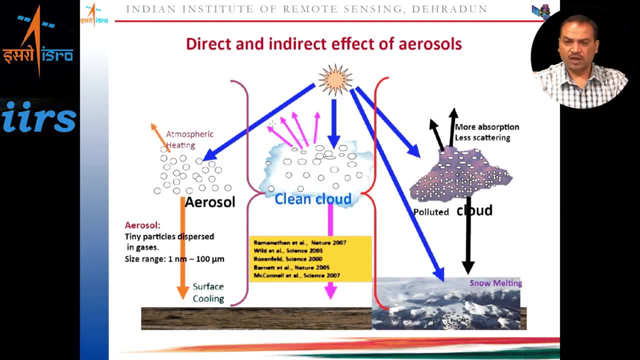 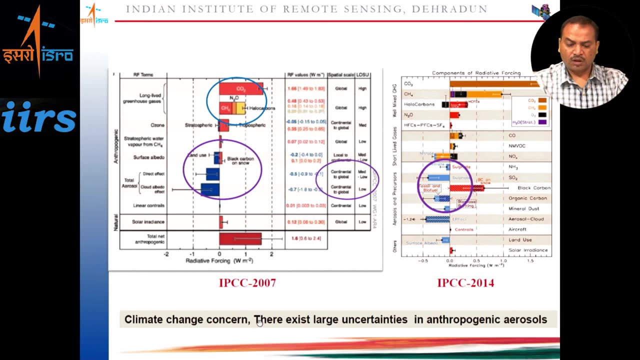 of liquid water content in the clouds. the particle size of the clouds can become smaller and it leads to the more scattering of the the sun radiation and thereby affecting the radiation budget. Now the, as you know, that IPCC, the internal panel of climate change- report of recent 2000. 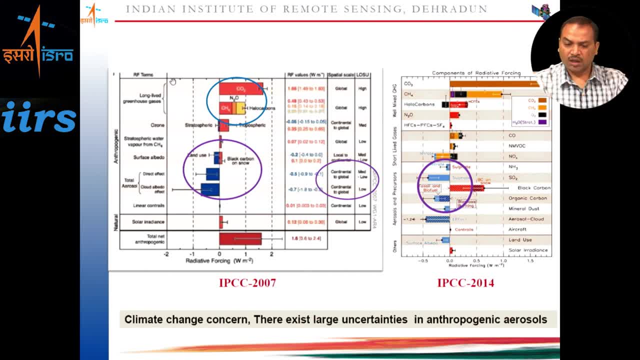 every 5 years. it comes 2014. now there is a. there is a wide acceptance that there is substantial amount of relative forcing due to the greenhouse gases. This is the greenhouse gases: there is a, carbon dioxide, nitrous oxide and the halocarbons. 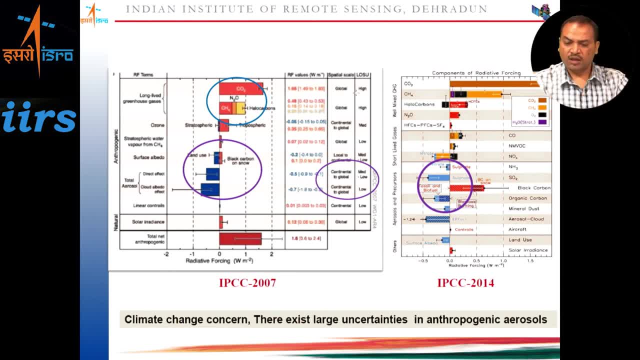 and if you see this, the column here, the, they are the, the the calculation of the estimation of the relative forcing. they have high confidence, the high high. Now, if you see here the, the aerosol relative forcing to, either due to the direct effect or the indirect effect, the, the confidence level is very low here it means because they. 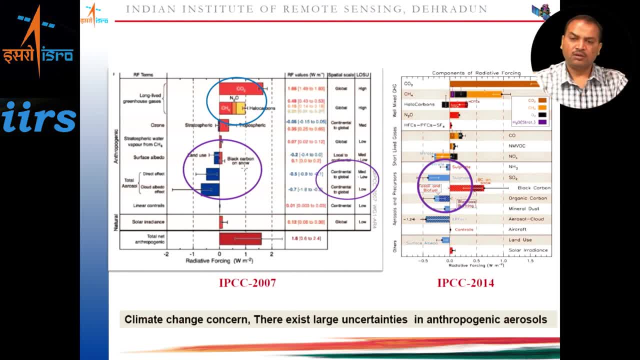 it is not very the, the, the measurements or the estimations does not substantiate with the ground measurement, lot of ground measurements, or due to the, the, the simulation studies, the model studies. So it requires more of frequent, more high temporal, high spatial data, either on the ground, 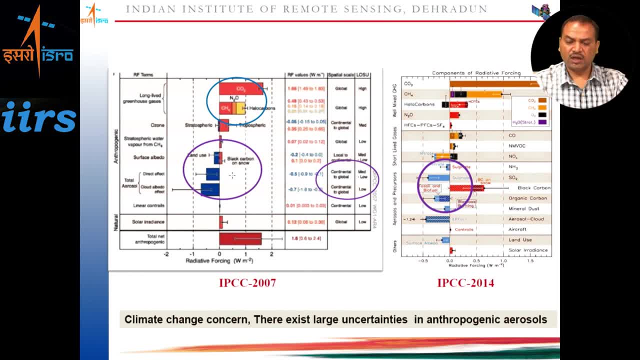 or through some sensors which can substantiate or which can help to have a high confidence level in the estimation of the relative forcing. and if you see the, the, the standard deviation is also quite high because of the, the. it tells about the type of the data, what the quality. 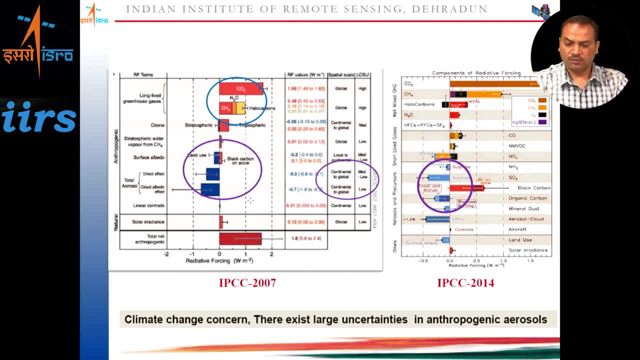 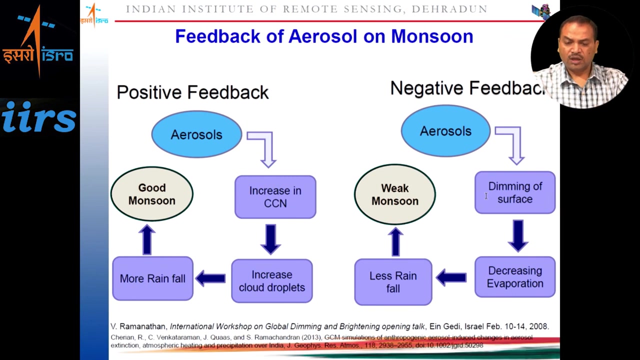 of the data being used for the estimation of the relative forcing In 2014.. The aerosol also has an affect on the monsoon, Uh, So it has an. it can have a positive effect as well as a negative affect. in terms of positive, 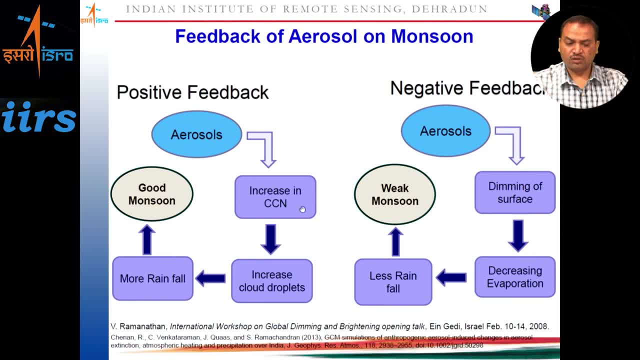 effect, as said, the more aerosol leads to, the more cloud condensation nuclei, So the increase in the cloud droplets, So they increase greater. so i think this one the veneration, the more it leads to and the more smaller the droplet from the coagular to the water. 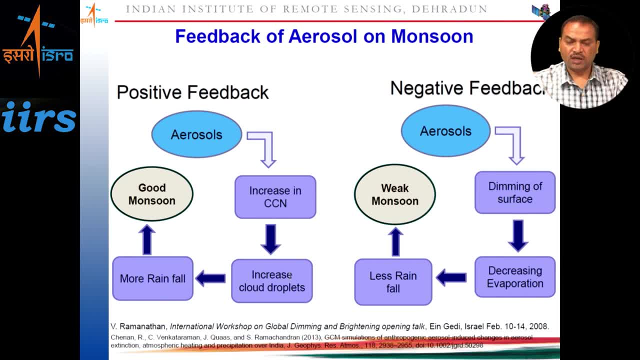 droplets. there are bigger, larger droplets, and then they settle down to the land in form of a rainfall. So more is the aerosols, more is the cloud condensation nuclei and more will be the rainfall. Another hypothesis is that it can have a negative feedback, meaning that many large aerosol 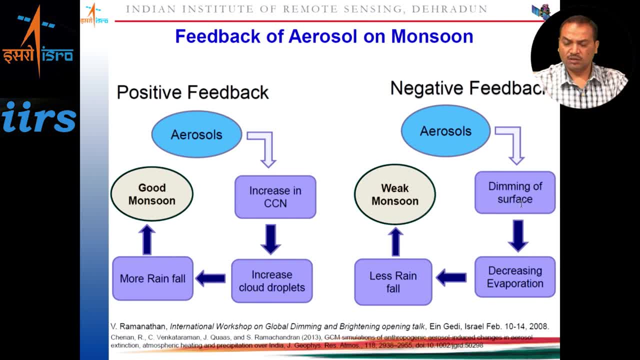 meaning the dimming of the solar radiation reaching over the surface, then decreasing the evaporation and less of the cloud formation, and which leads to the less of rainfall and weakening of the monsoon processes. So sometimes we are not knowing exactly what is the process happening, whether it is a positive 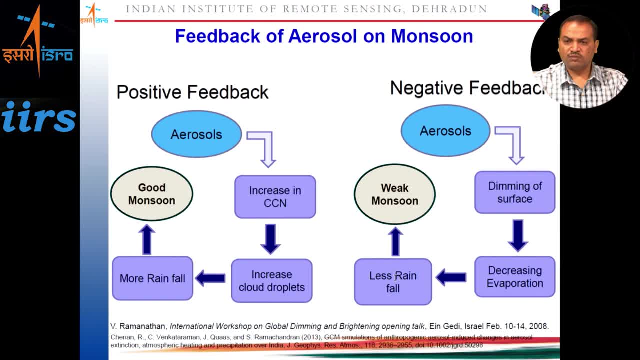 feedback, whether it is a negative feedback. There are many studies which shows both this feedback that somewhere says that the aerosols are having for so many decades having the more of rainfall. Some have says that there, the over the regions, there is scarcity of The rainfall and the monsoon chain has the weakened and the process has become diminished. 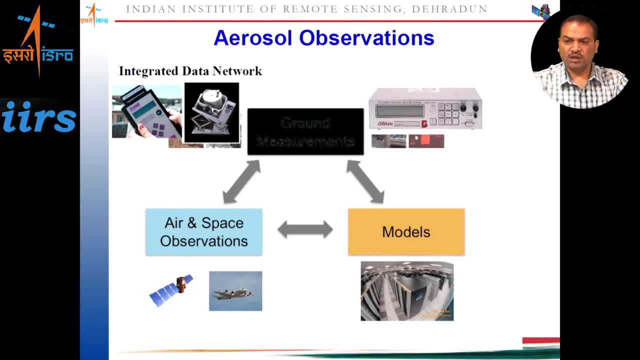 So, as I said, the, to increase the confidence level of the level of understanding in terms of the properties of the aerosol, whether it is a physical property, the optical or the relative property, one needs to have a consolidated, integrated and cohesive aerosol studies in terms of data collection, very local and regional scales, either in 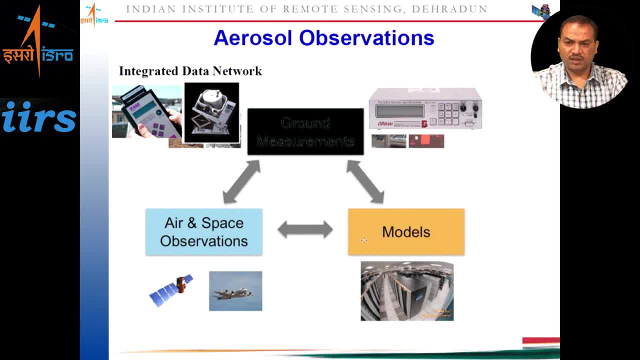 terms of the ground measurements or from a sensors in the sky, that is, the satellite observations. So in this, the and also this combination of these two can also help in the formation of the simulation, simulation data, data, and then it can help in the models to perform. 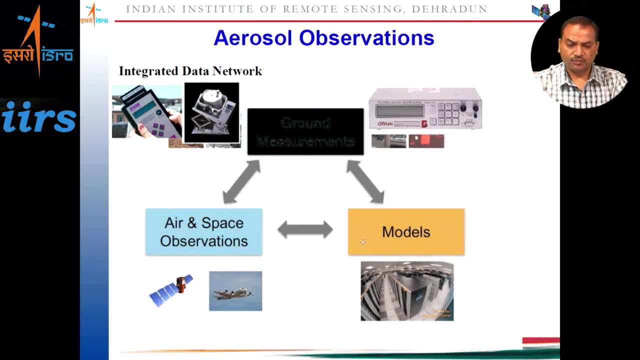 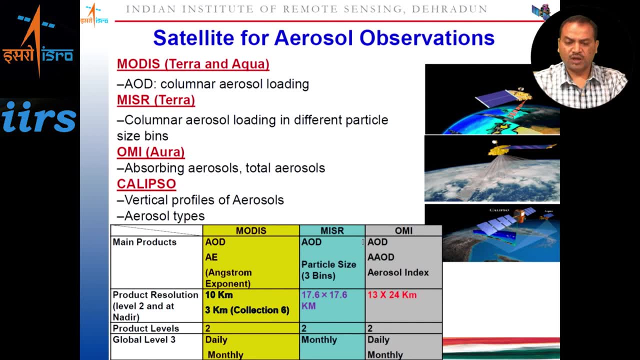 at a regional Level and a global level. Coming to the, the satellite observation, which are helpful for the aerosol studies. Modest is one such satellite which provides data. they come up with a lot of products over the aerosol optical depth, which is an optical parameter, and also there are other optical